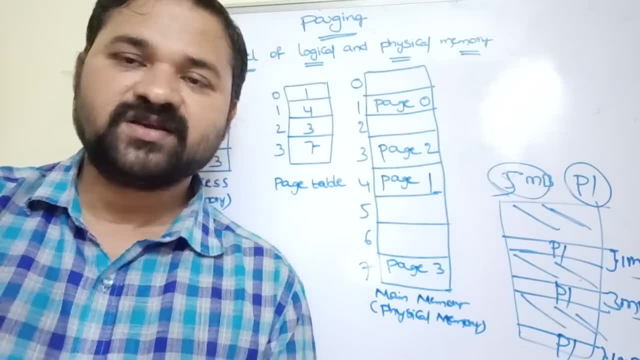 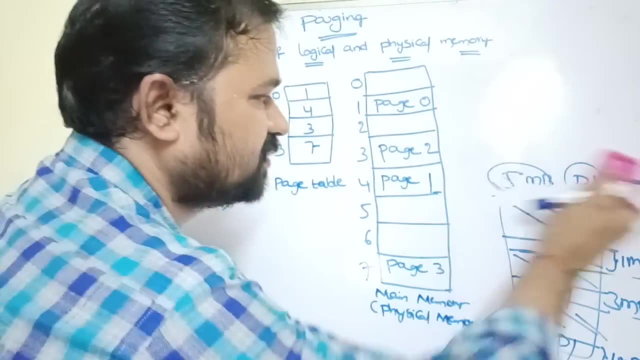 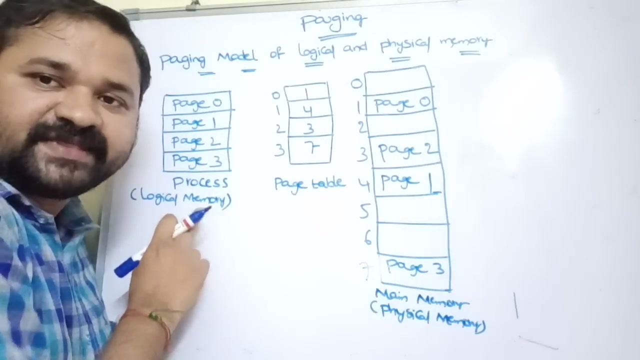 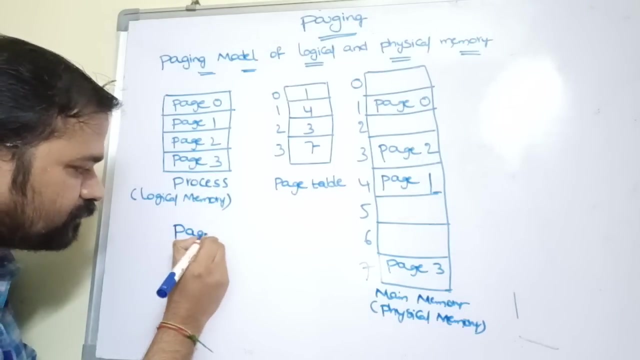 So this is nothing but non-contiguous memory allocation. So wherever there is a free space, then operating system can make use of that free space for storing the process. So let us see how paging will be implemented. In paging, the process is divided into a number of partitions called pages. The size of each page must be same. 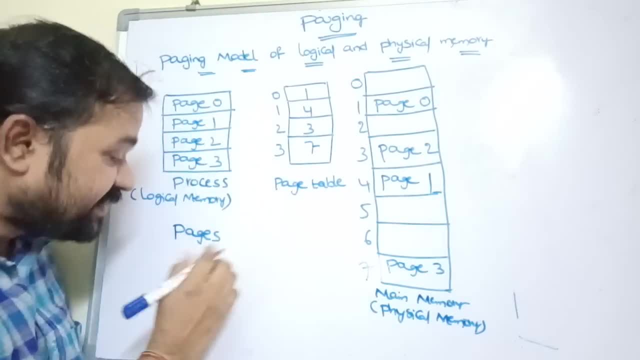 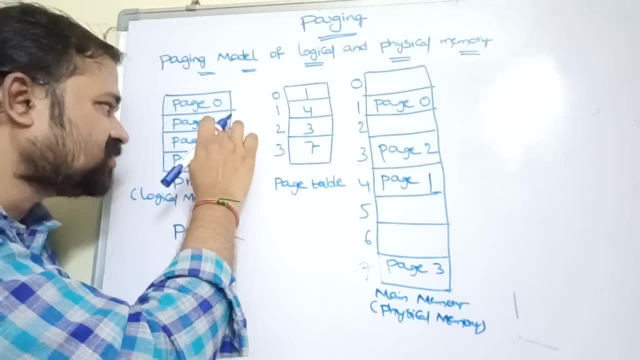 That means if page 0 size is 1 KB, then the remaining pages size is also 1 KB. So page 1 size is also 1 KB. page 2 is also 1 KB. page 3 size is also 1 KB. 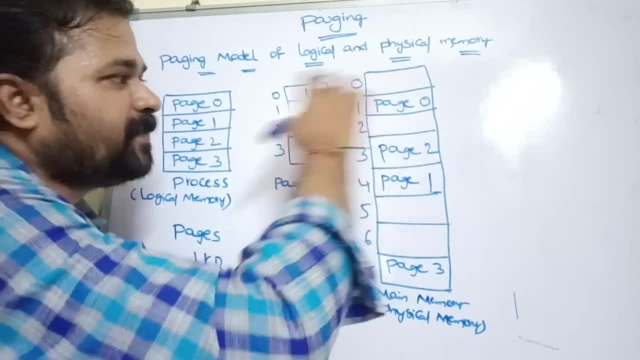 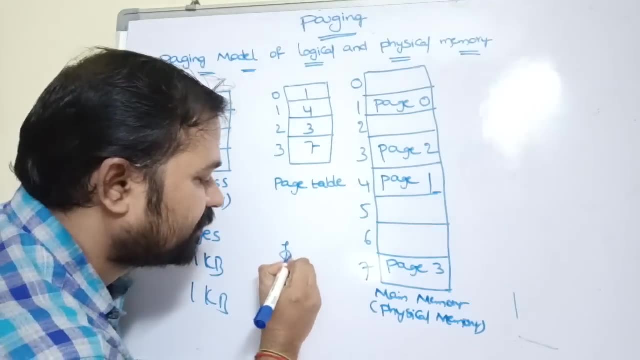 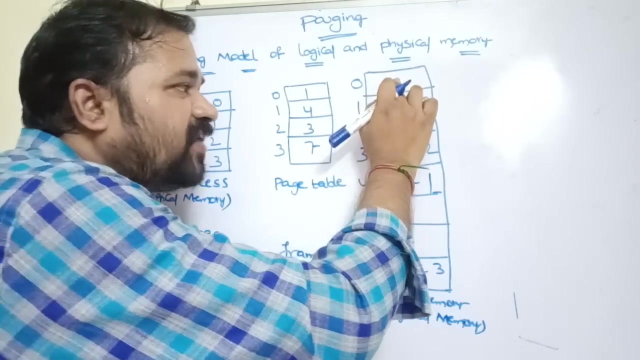 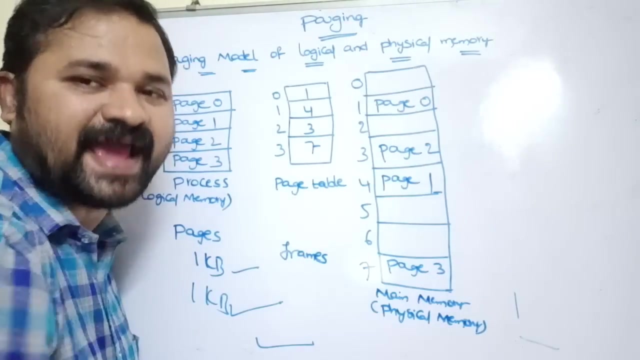 Next. this is nothing but our main memory. Main memory is also divided into a number of partitions called frames. Here the size of each frame must be same. That means if frame 1, if first frame size is 1 KB, then the second frame size is also 1 KB. third frame size is also 1 KB, like that. 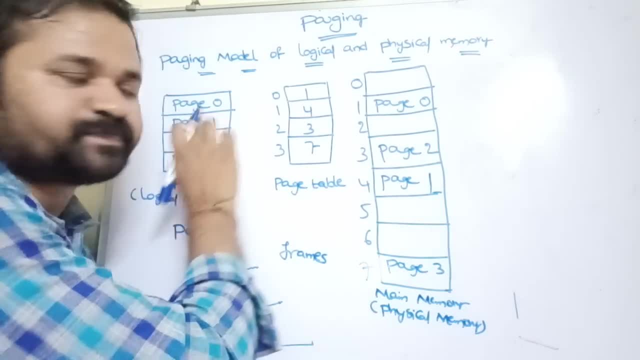 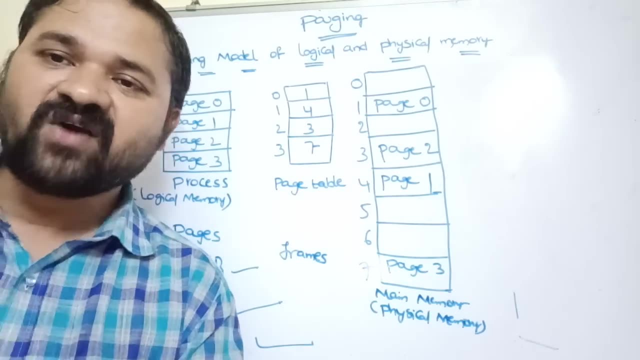 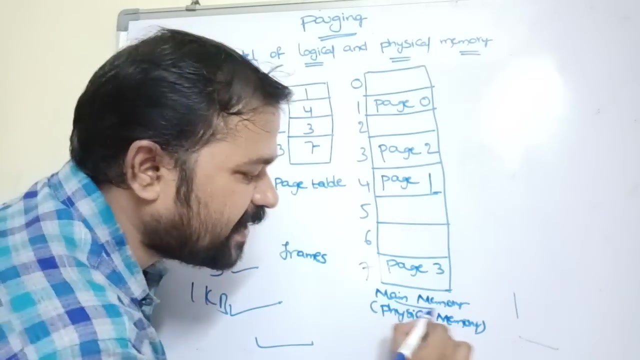 And one more point here is: the page size and frame size must be equal. Page size and frame size must be equal. So here we have 3 points. First point: this is process. Process means logical memory. This is main memory. Main memory is nothing but physical memory. 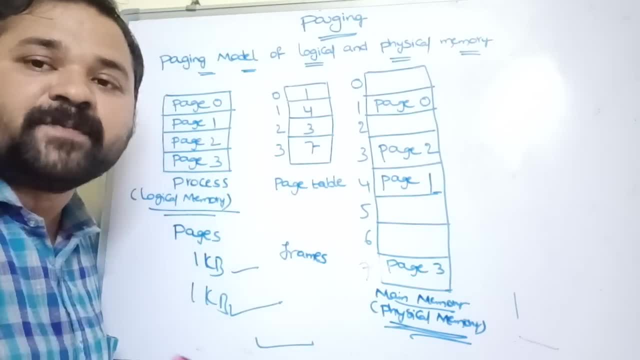 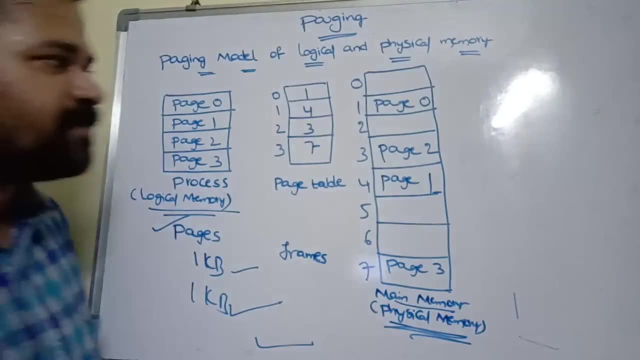 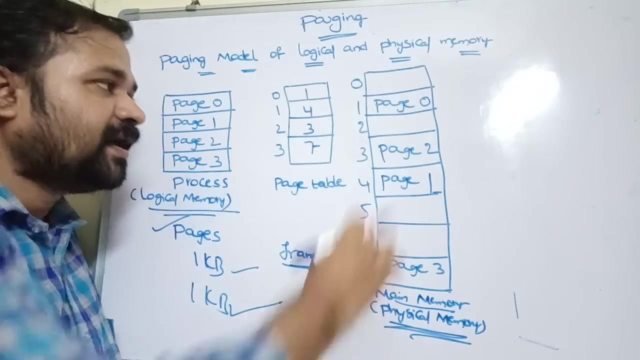 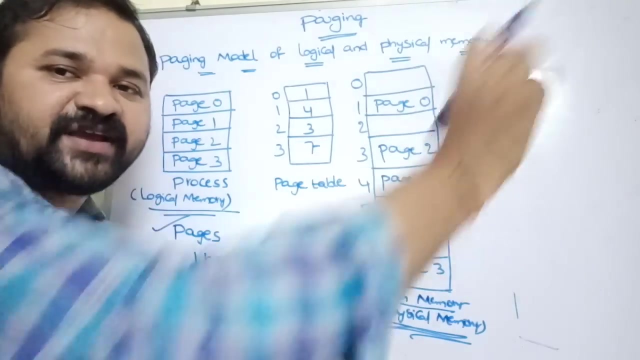 If process is divided into a number of partitions called pages, and the size of each page must be same. only- Second point, main memory is divided into a number of partitions called frames, and the size of each frame must be same. If frame 1 size is 1 KB, then frame 2 size is also 1 KB. frame 3 size is also 1 KB, like that. 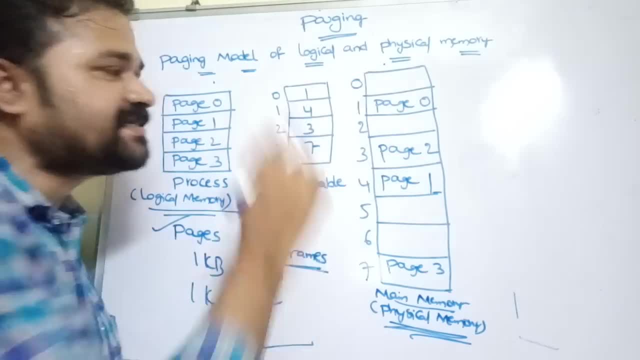 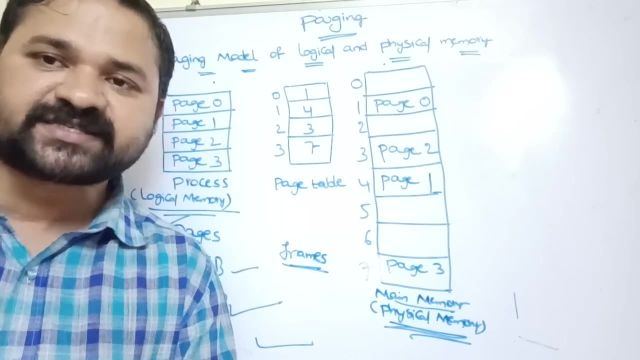 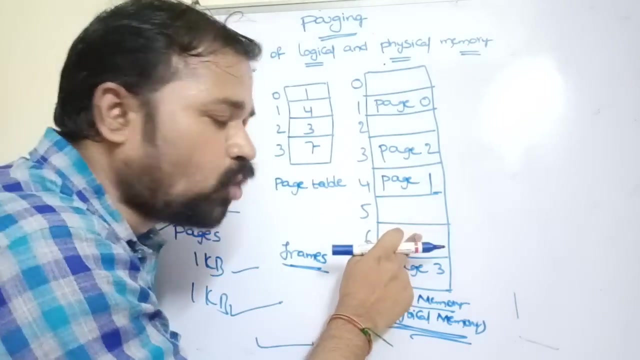 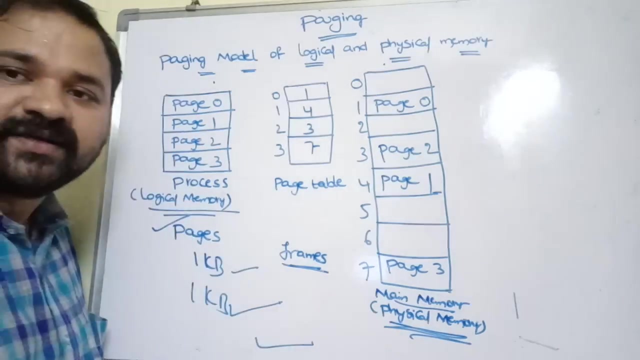 Next point: page height, frame size must be same. next, whenever cpu needs to execute a process, then the pages of the process from the secondary memory are loaded into frames of the main memory. so this is our process. so we know that the process is divided into a number of equal size partitions. 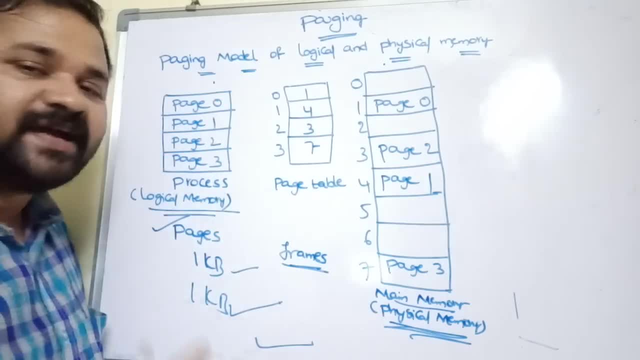 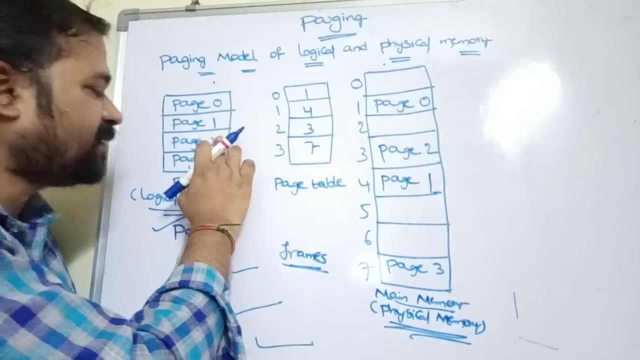 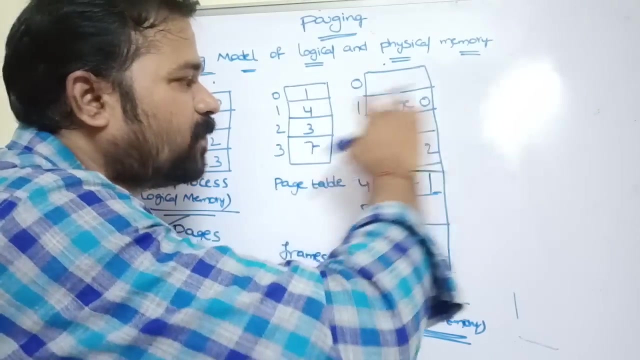 called pages. so this is our process. let our process contains four pages where the first page is page zero, second page, space one. second, third base, page two, fourth page pay three like that. so this is our main memory. so the main memory is divided into a number of equal size partitions. 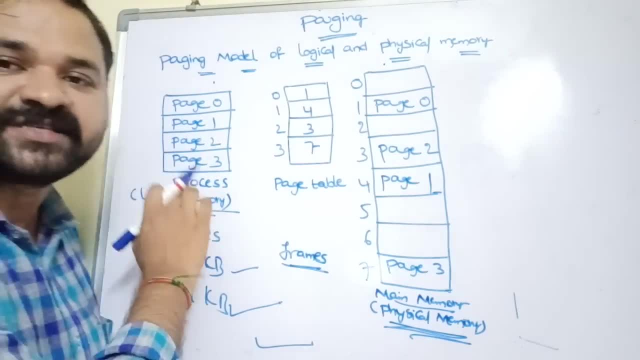 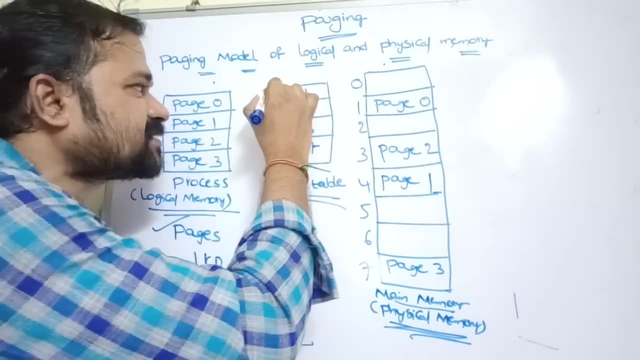 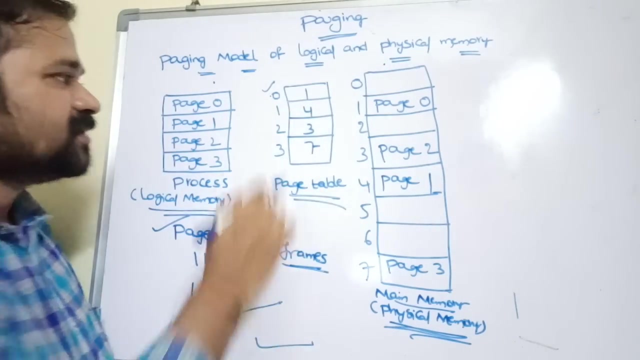 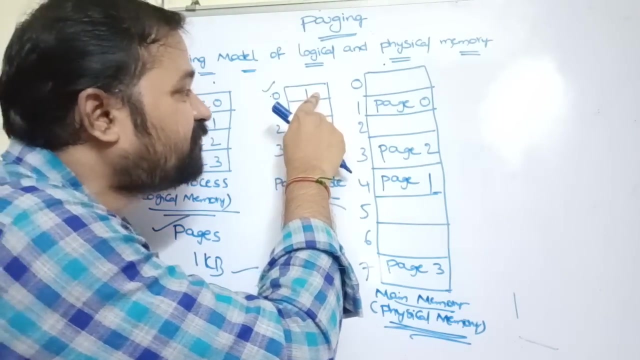 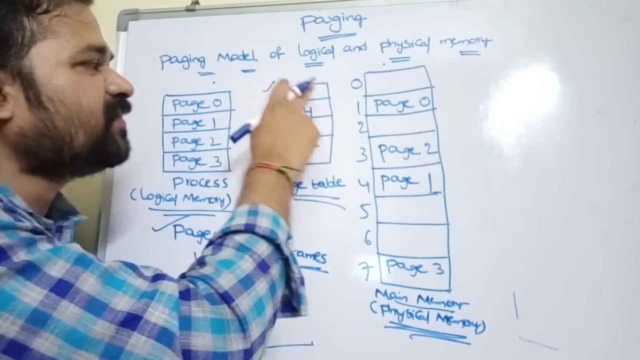 called frames. okay, this frame size and page size should be same. next, this is nothing but pasteable. pasteable. pasteable acts is available in frame number one. so these are nothing but frame numbers. zero, one, two, three, these are nothing but frame numbers. so page number zero is available in frame number one. so this frame 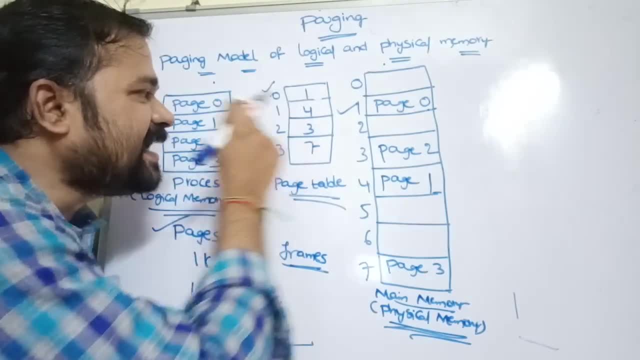 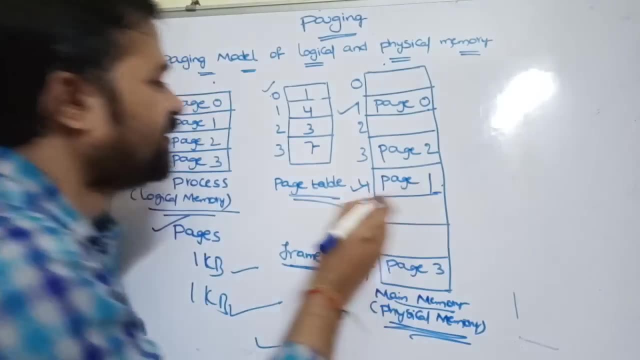 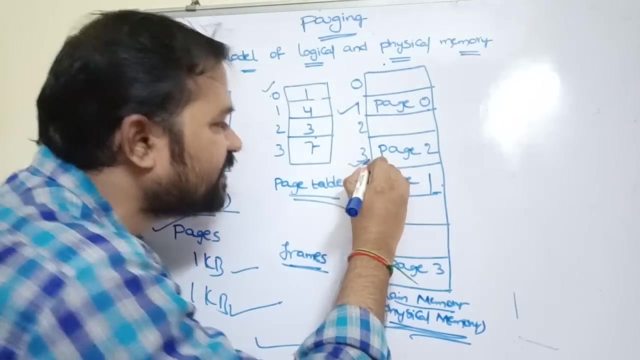 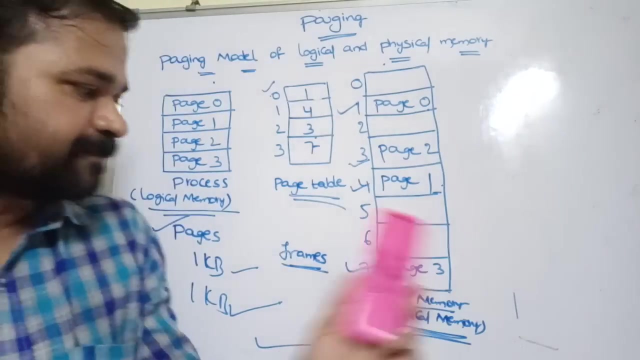 number one contains page zero. next, this second line specifies that page one is available in frame four, so fourth frame contains page one. this line specifies that page two is available in frame three, so frame three contains page two. so this line specifies that page three is available in frame seven, so frame seven contains page three. now let's see paging hardware. 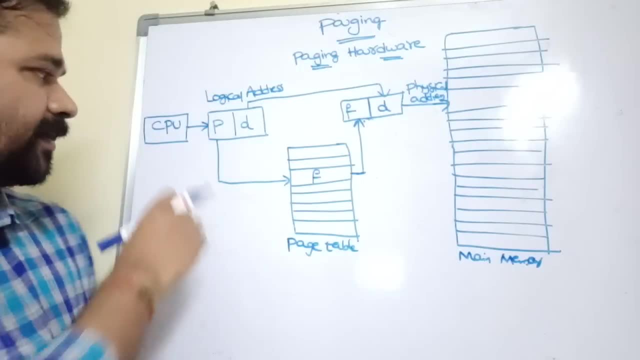 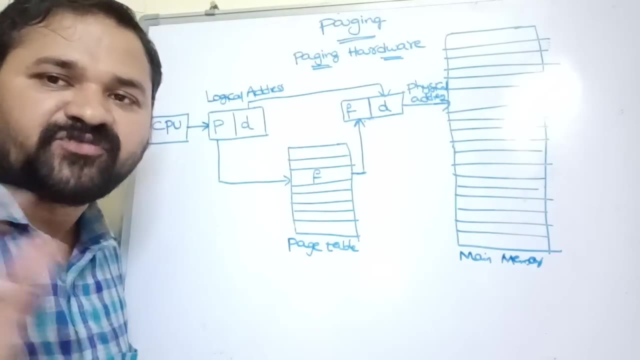 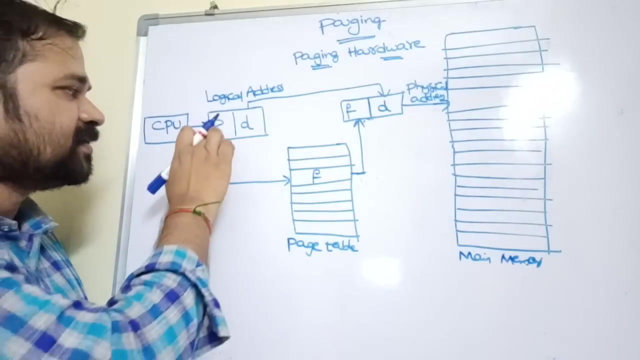 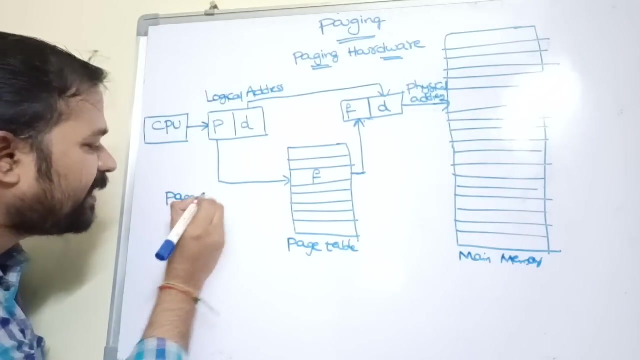 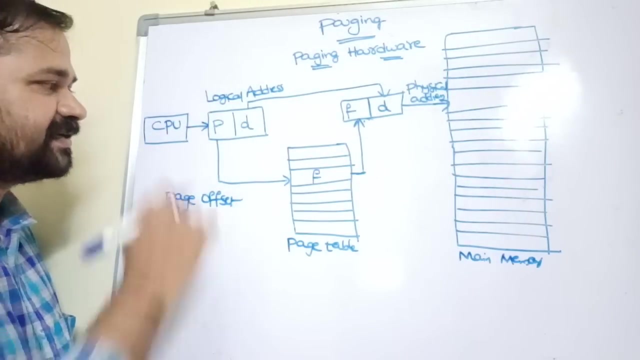 paging hardware. in order to execute any instruction, cpu generates logical address for the corresponding instruction. logical address is mainly divided into two parts. the first part specifies page number. the second part specifies: b means page offset. so what is the first part, page number. second part: page offset. here d stands for displacement. so page offset is nothing but displacement. 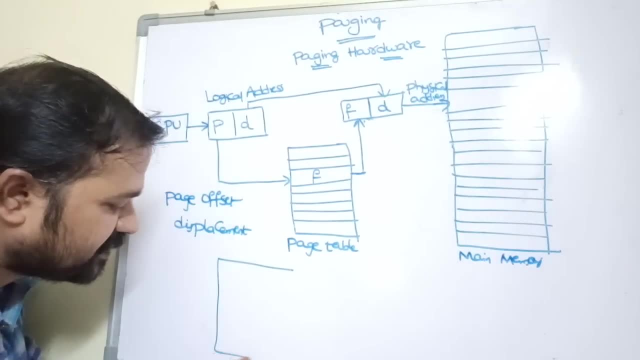 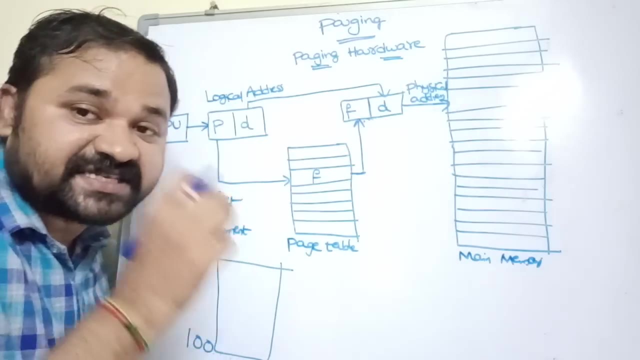 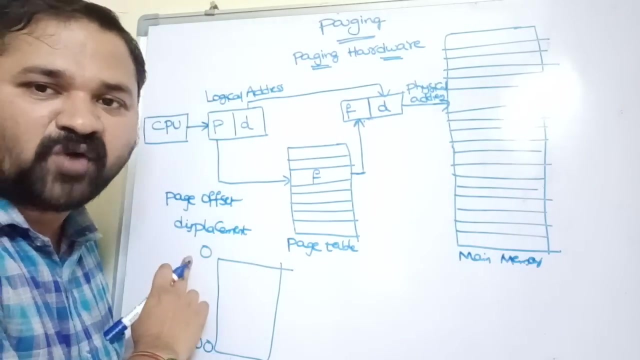 so let we have a page like this. let this page contains 100 locations. so this is nothing but displacement. so which instruction we are accessing? let we are accessing the first instruction of the base, so displacement or offset is 0. let we want to access first instruction, then the displacement. 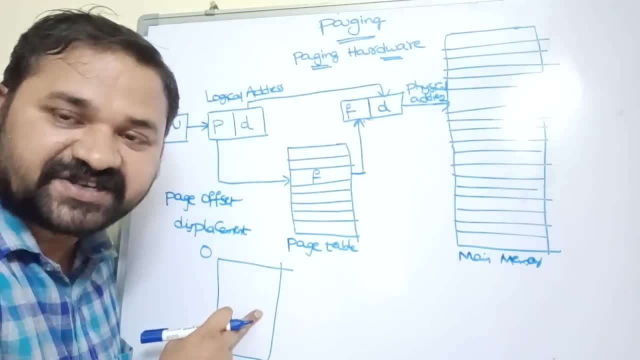 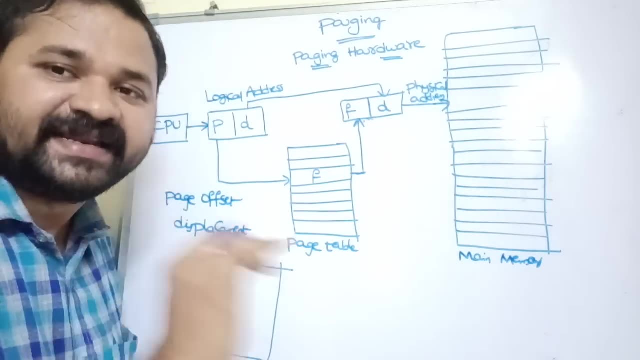 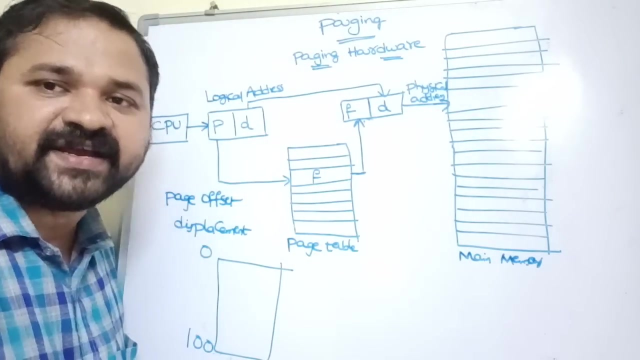 or offset is 1, let we want to access 10th instruction. then displacement or offset is 9, so like that. so see, in order to execute any instruction, cpu generates logical address. here the logical address is divided into two parts. the first part specifies page number. 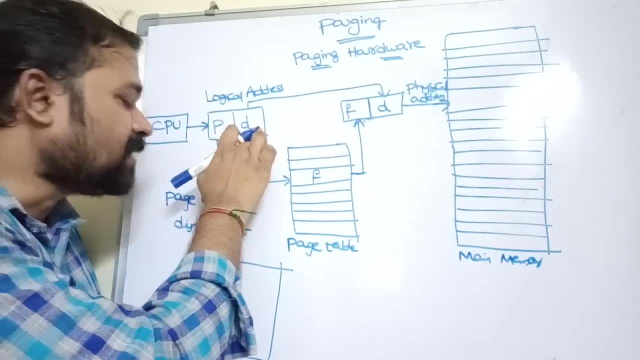 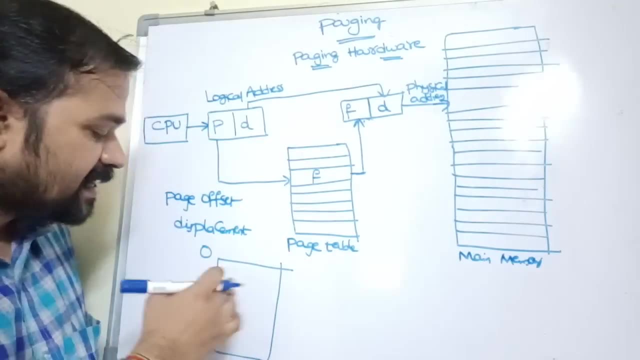 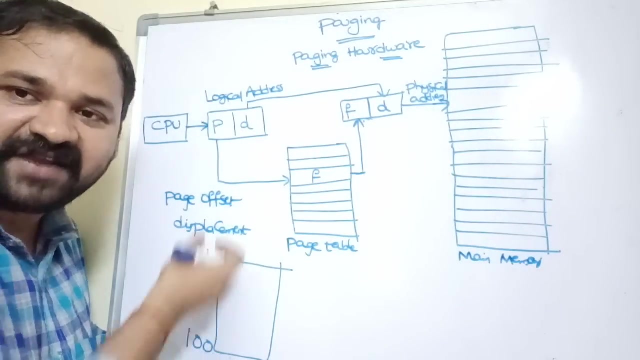 page number is denoted with p. the second part specifies page offset. page offset means displacement. displacement means line number within the page, location within the page. so let we have 100 elements, let we have 100 instructions in the page. so, in order to access the first, 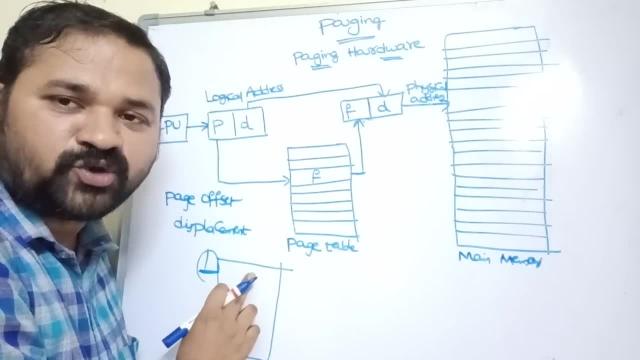 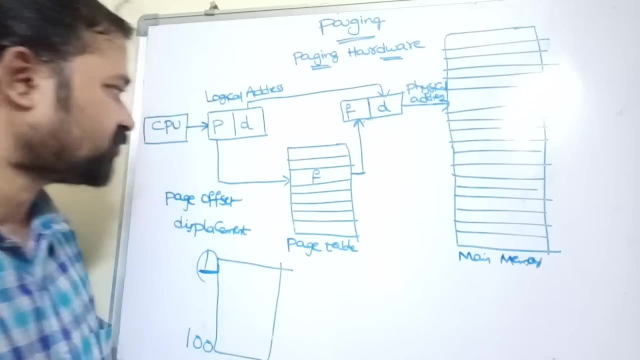 instruction. here the offset is 1. so if you want to access the second instruction, then offset is 2. if you want to access the second instruction, then offset is 2. if you want to access the second instruction, then offset is 10, like that. okay, this page number will be given as input to the 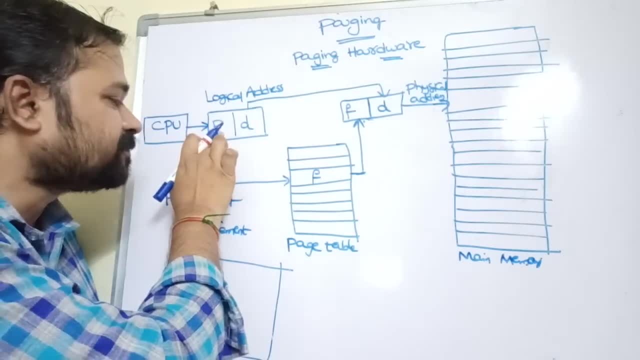 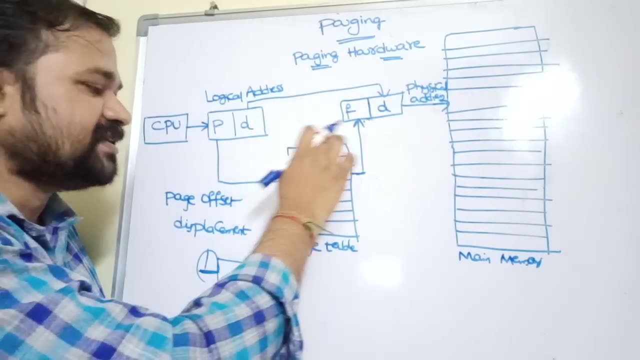 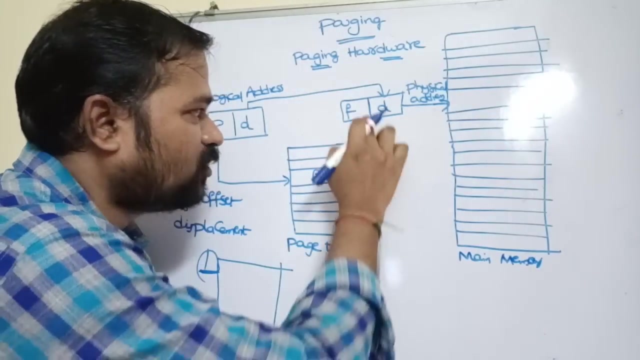 page table. page table accepts page number as the input and it produces frame number as the output. so this is page table. so page table is accepting page number as the input and it is producing frame number as the output. here f stands for frame number. if we combine frame number with the input, 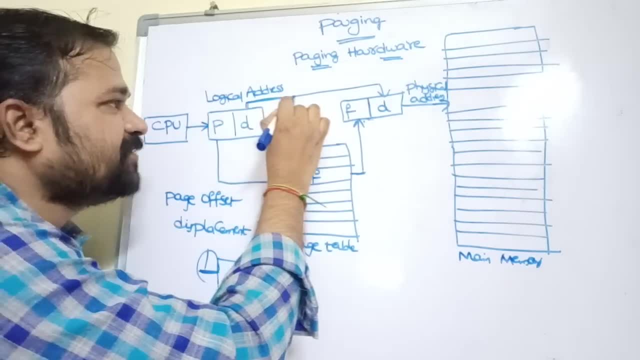 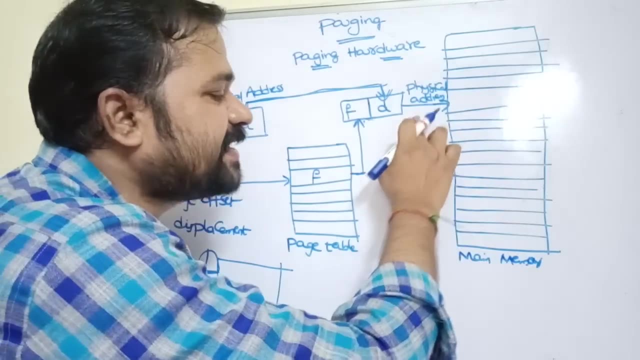 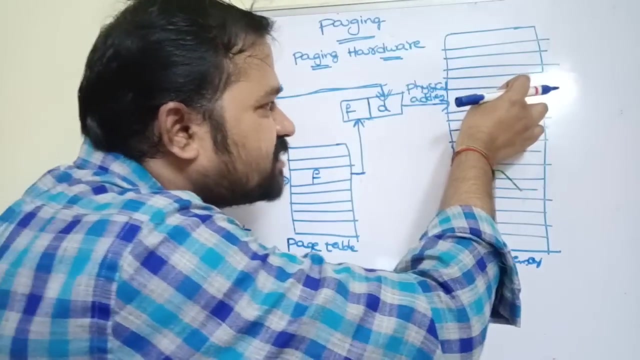 here f stands for frame number as the input and it is producing frame number as the output. if we combine frame number with the offset, then it gives the exact physical address in the main memory so that cpu executes the corresponding instruction which is available at this address. so here we have two addresses: logical address. 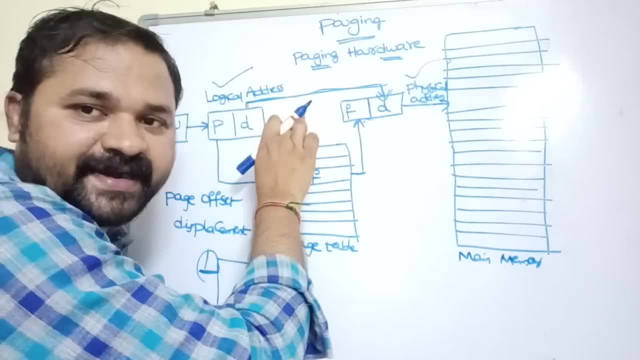 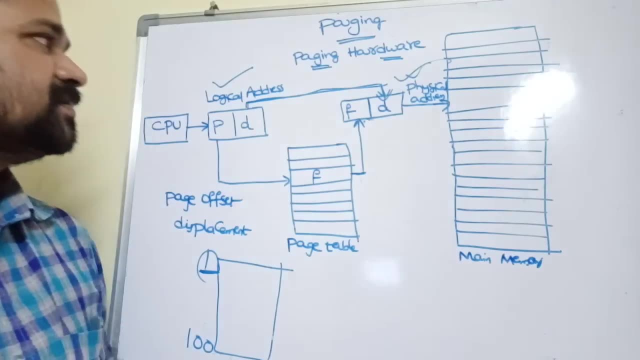 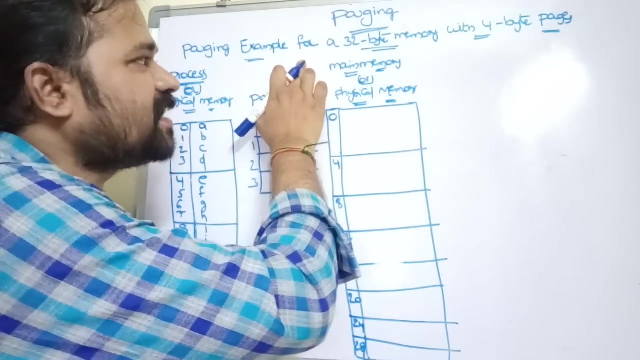 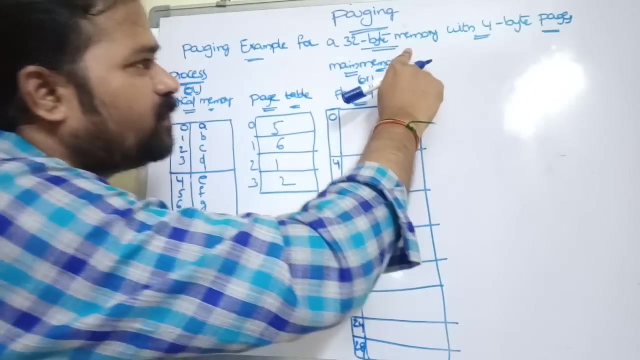 physical address. logical address means the address generated by the cpu. various physical address means the address generated by the main memory. so this is about paging hardware. now let's see this example- paging example for a 32 byte memory with 4 byte pages. so the size of the main memory is 32 byte, 32 bytes and the size of a process, the size of a page, is 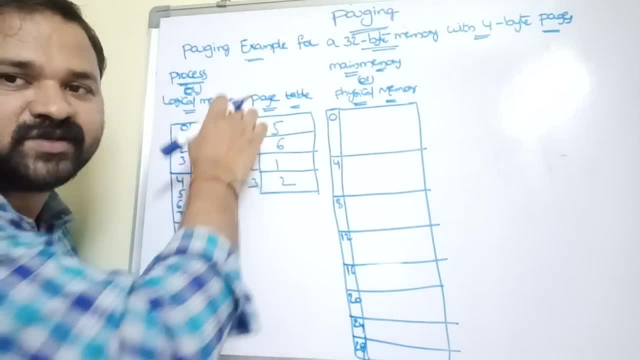 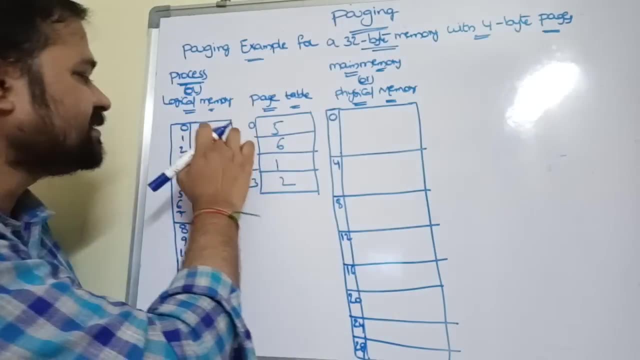 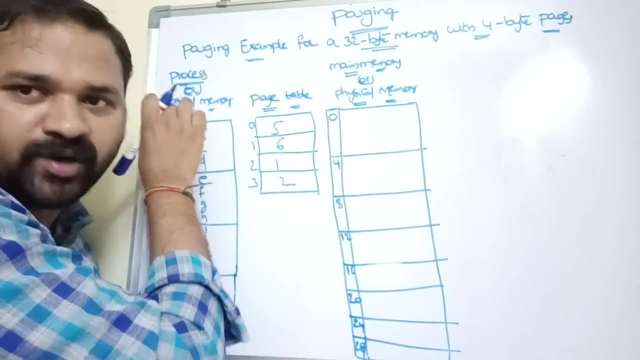 4 bytes. so this is our process, or logical memory. so we know that the process is divided into a number of partitions called pages. here the size of a page is 4 bytes. so the size of a frame will also becomes 4 bytes. why? because we have to load the page into the frame. okay, so the size of the 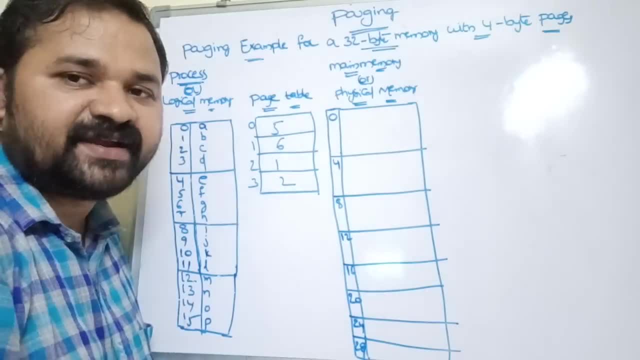 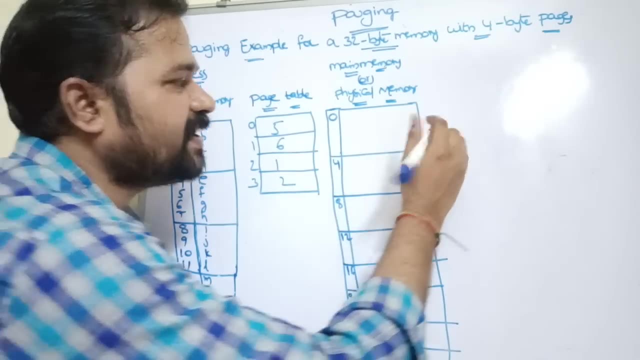 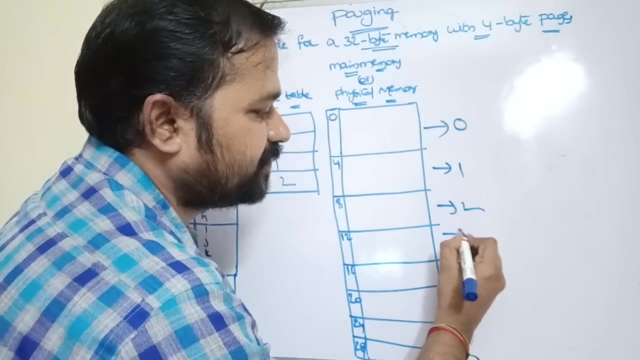 main memory is 32 bytes, so main memory is also divided into a number of partitions, called frames, where the size of a frame is what? four bytes, so four into totally we have eight frames here. so this is, uh, zeroth frame, first frame, second frame, third frame, fourth frame, fifth frame, this is sixth frame and this is nothing but seventh. 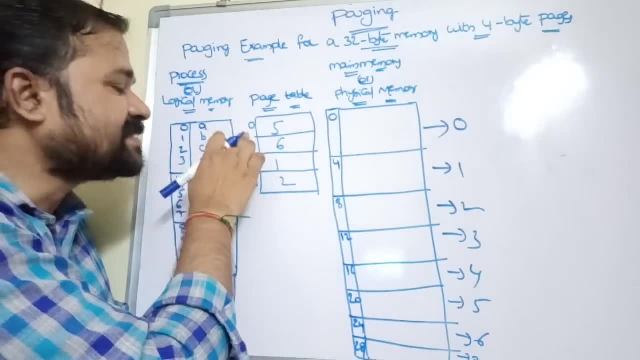 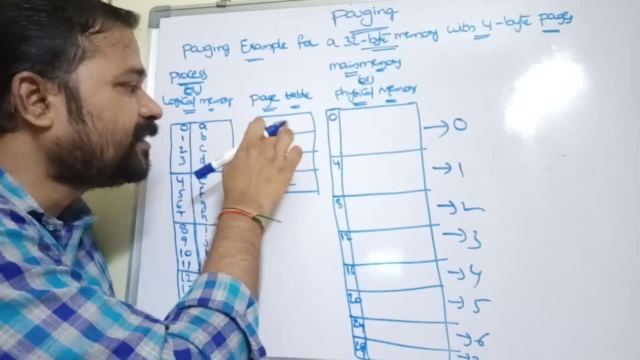 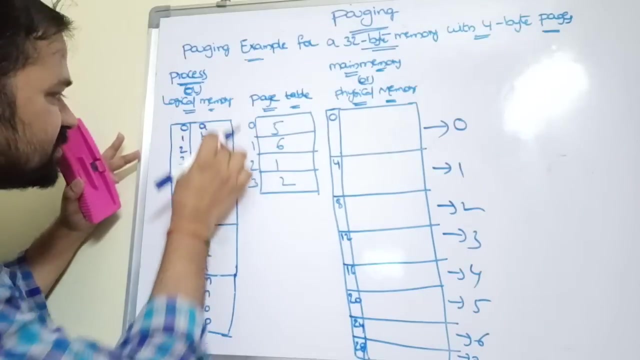 frame. so this page map table specifies the page number and the corresponding frame number output. so here it specifies that page number 0 is stored in frame number 5. so this is frame number 5. so what is space 0? this is page 0. so what is the content of page 0? a, b, c, v. so first location, instruction a. 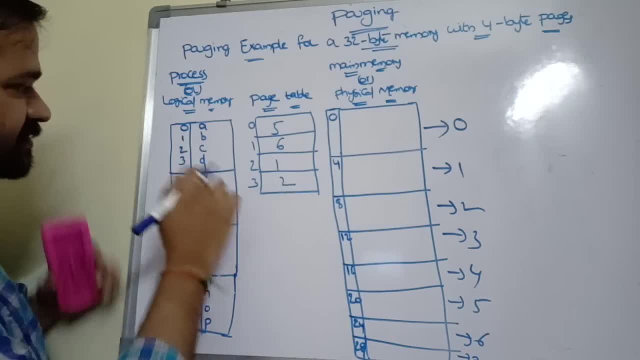 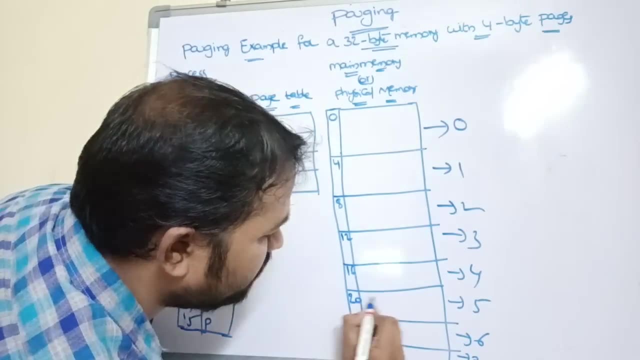 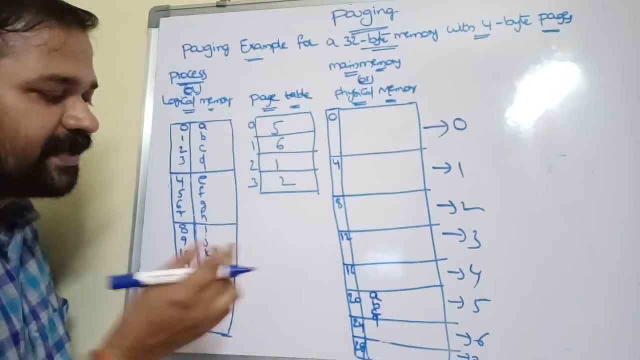 second offset, instruction b, next offset c, like that. okay, so in which space, in which frame? we have page 0 in fifth frame. so this is fifth frame. so in 20 we have to store a in 21, b in 22, c, next 50. okay, here, if you want, we can calculate the physical address with the help of a formula. 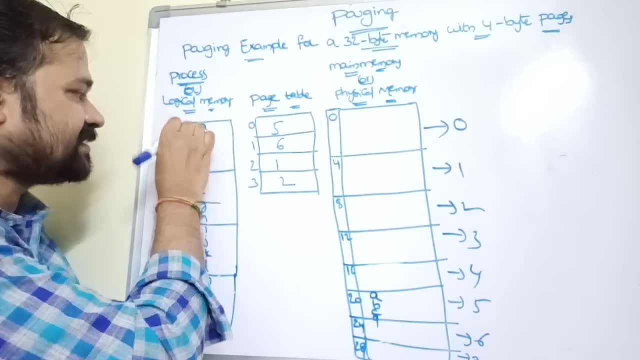 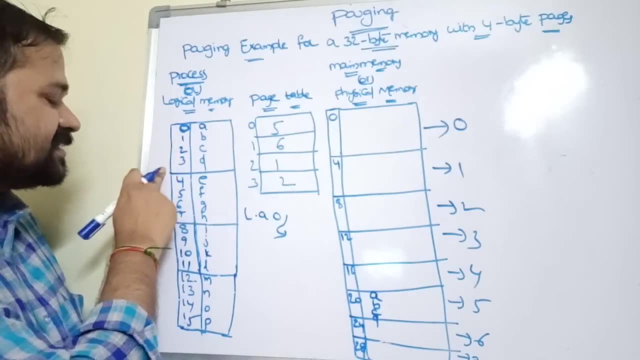 here, if you take the first instruction, if you take the first logical address, that is zero. here the logical address is zero. so what is zero here? zero means this is zeroth space, so pace: 0. so what is the offset here? this is nothing but zeroth offset. 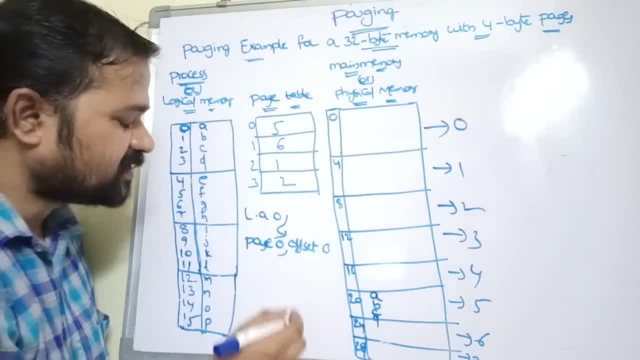 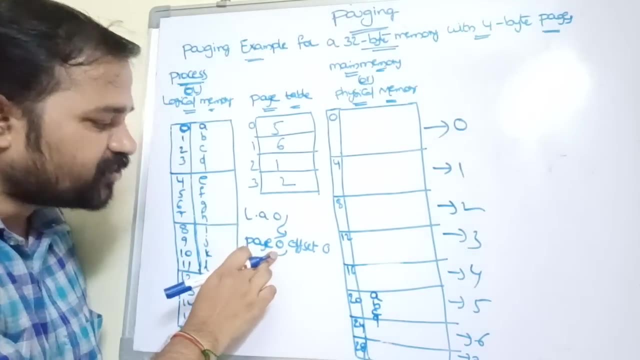 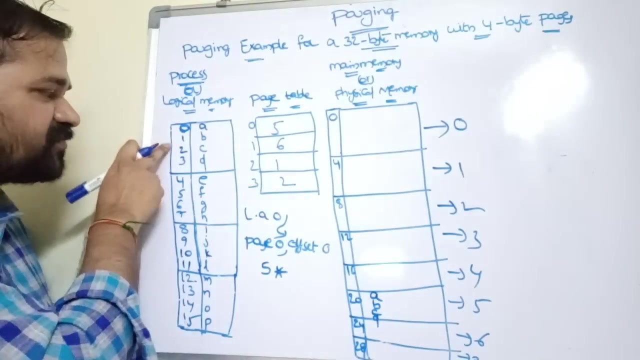 so offset is also 0. so here the formula is very, very simple. we have to check in which frame the corresponding page is available. so this is space 0. so page 0 is available in frame 2.. 5 so 5 into. so what is the size of a page? the size of a page is 4 bytes. so 5 into 4 plus what is the? 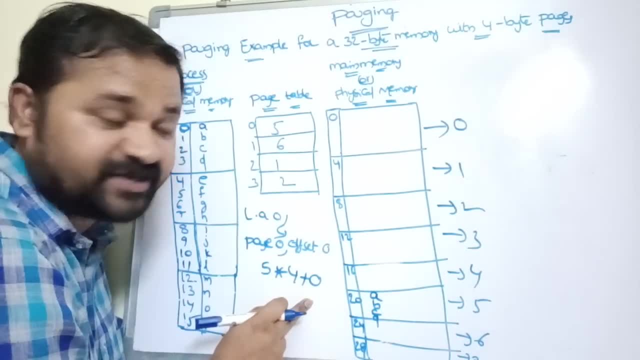 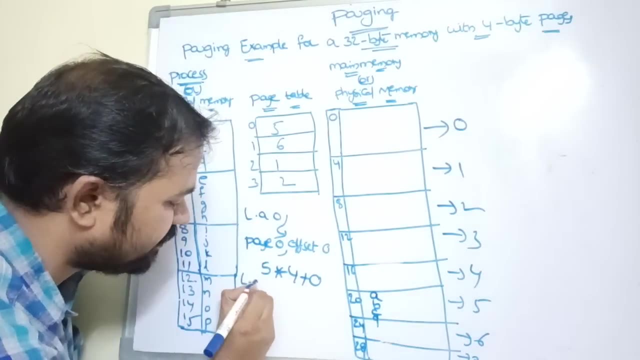 offset here 0, so 5 into 4, 20, so 20 plus 0, 20, so in 20 we have a. if you take the next instruction, that is 1 logical address 1. okay, so what is logical address 1? this is nothing but page 0 only. 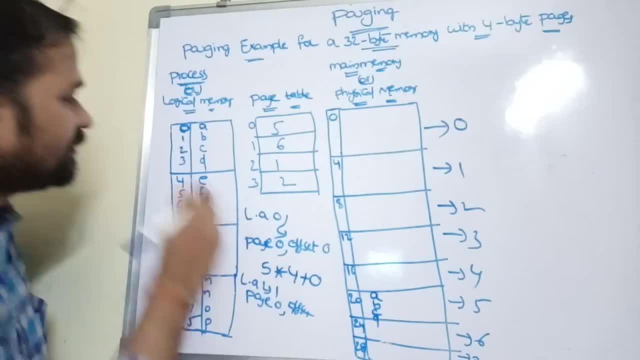 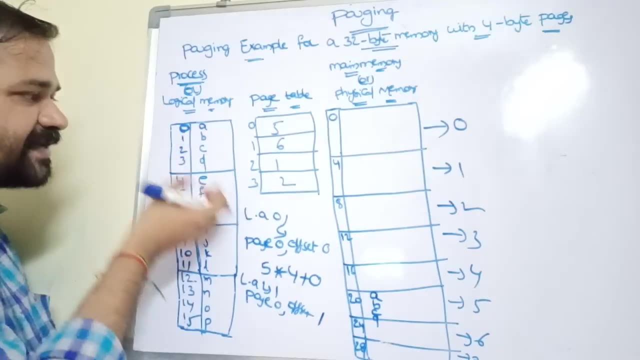 but what is the offset here? here the offset is 1. 0 means offset 0, 1 means offset 1. okay, so we know that page 0 is stored in 5. so 5 into what is the size of your page? 4 bytes plus what? 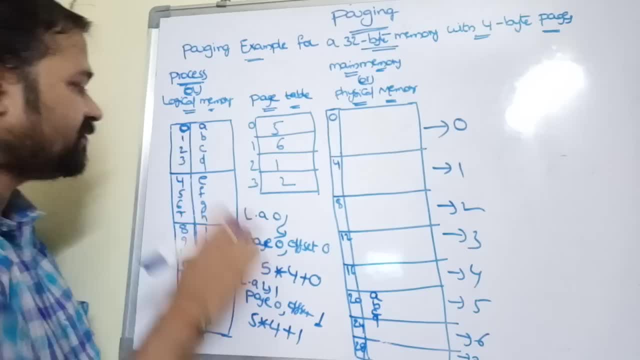 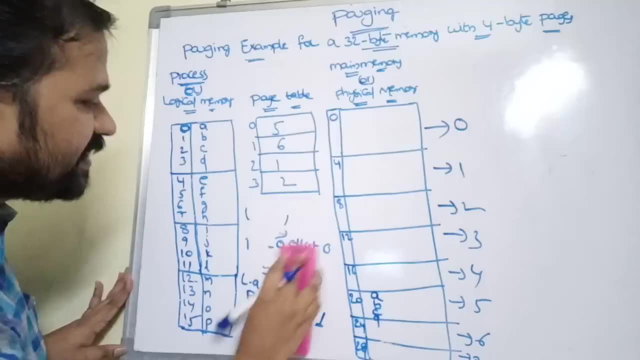 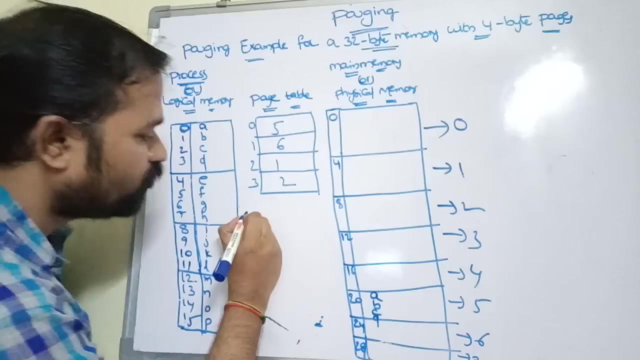 is the offset here? 1, so 5 into 4, 20, 20 plus 1, 21. so in 21 physical address we have to store b here, okay, so likewise c and d will also be stored. let us take the next one. if you take the next byte, that is 4. so what is 4 here? 4 means it is page 0, and what is the offset? 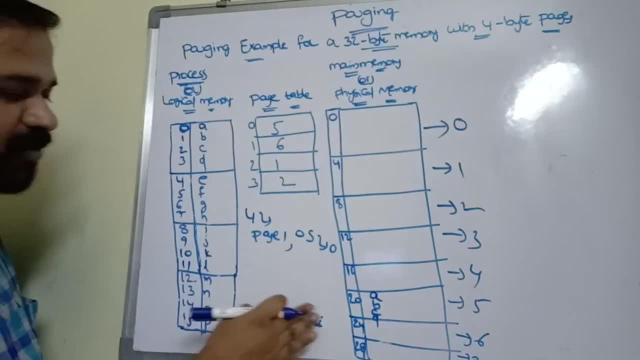 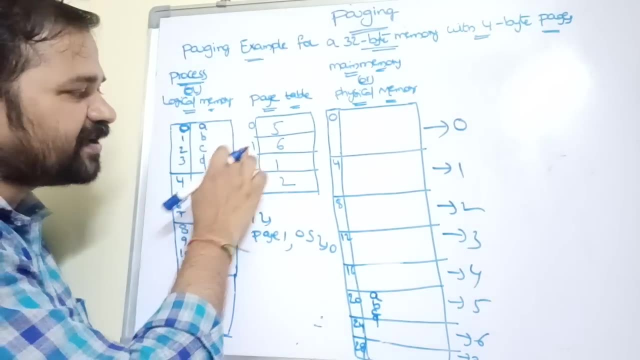 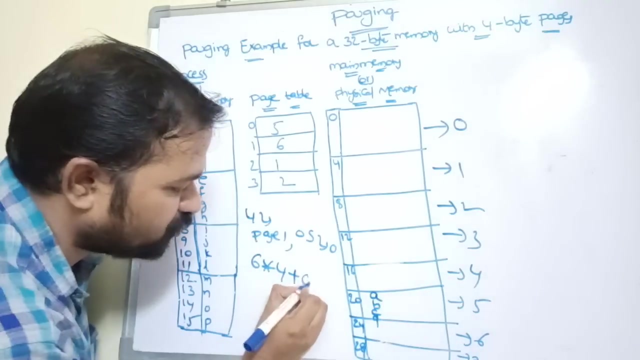 here offset is 0. so if you want to calculate the physical address, then what is the formula here? 4 is nothing but page number 1. page number 1 is available in frame number 6, so 6 into size of your page, 4 bytes plus. what is the offset here? 0 so 6 into 4, 24, so 24 plus 0. 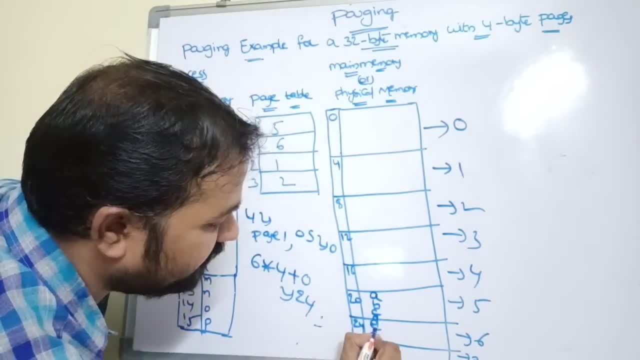 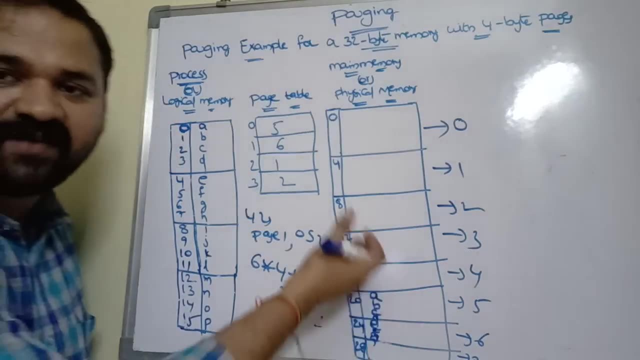 So in 24, we have to store E. In 25, we have to store 5.. In 26 address we have to store G. In 27 address we have to store 8.. So likewise we have to calculate physical address for the corresponding logical address. 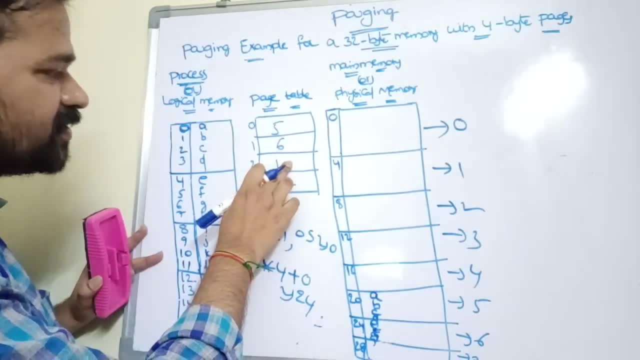 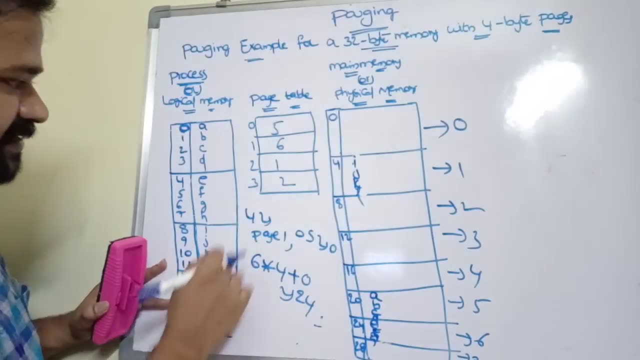 Next, if you take page number 2, page number 2 is available in frame number 1.. So this is frame number 1.. So IJKN. Next, this is nothing but page number 3.. So page number 3 is available in frame number 2.. 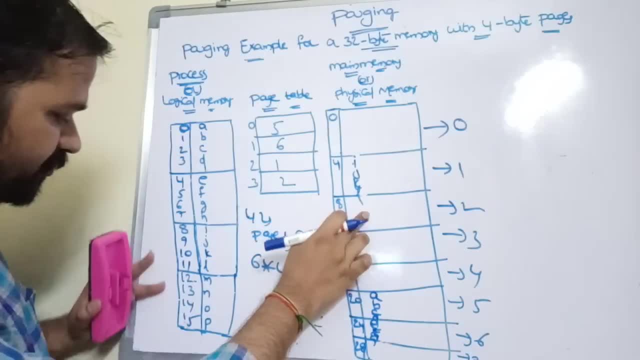 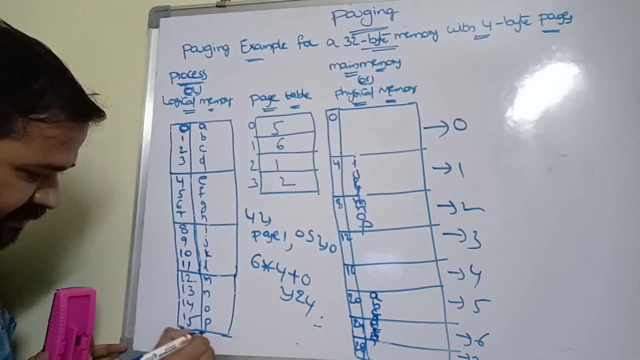 Page number 3 is available in frame number 2.. So this is frame number 2.. So in frame number 2, we have to store MNOP. So here what is P? here P means, let us calculate the physical address for this 15.. 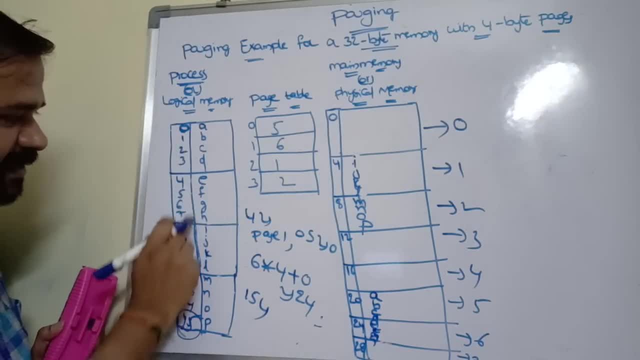 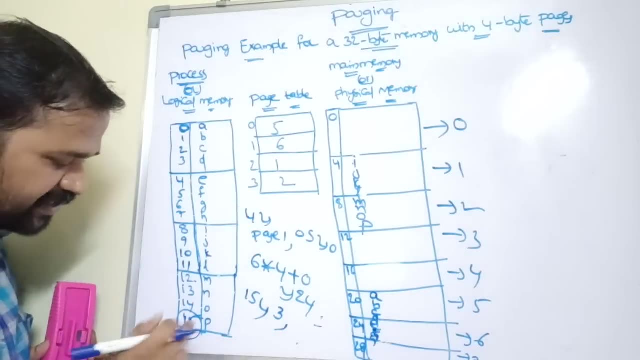 So what is 15 here? 15 means page number. this is 0,, 1,, 2, 3.. So page number 3, what is the offset here? 0,, 1,, 2, 3.. 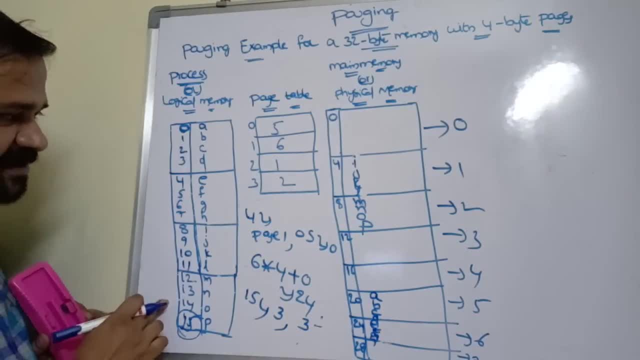 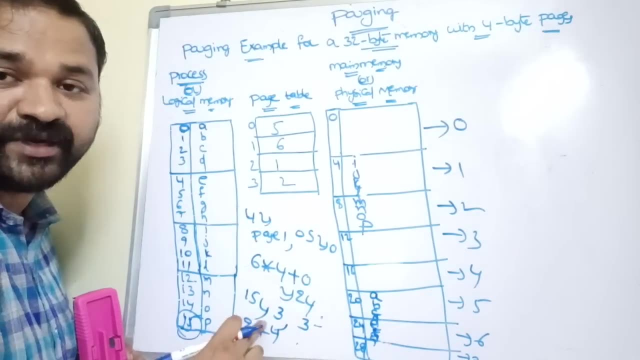 Offset. Offset is also 3 here. So this is start page. Start page is available in frame number 2.. So 2 into what is the size of page? 4 bytes. So 2 into 4 plus what is the offset here. 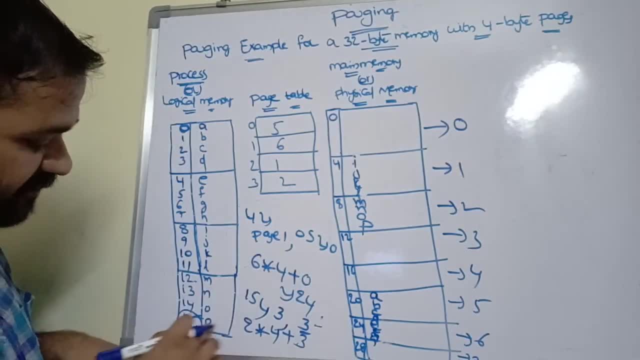 3. So 2 into 4, 8. 8 plus 3 means 11.. So in 11, physical address we have to store P. So this is nothing but 11. So in 11, we have to store P. 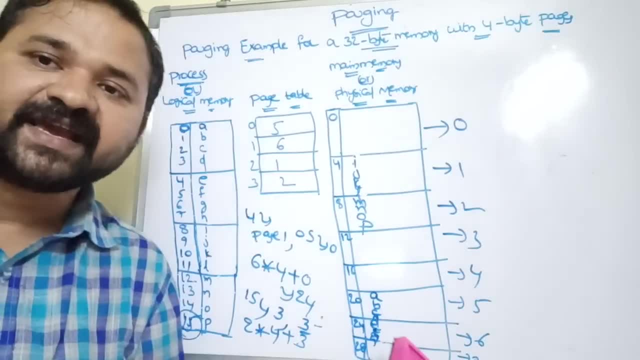 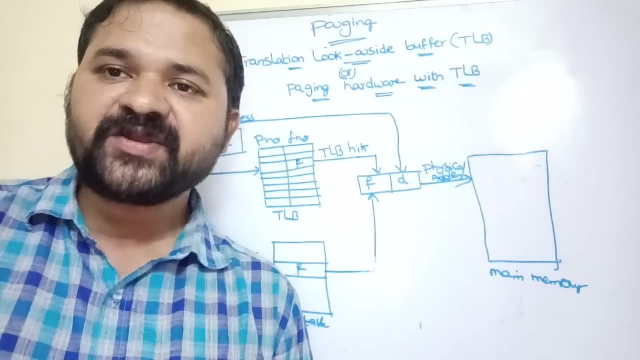 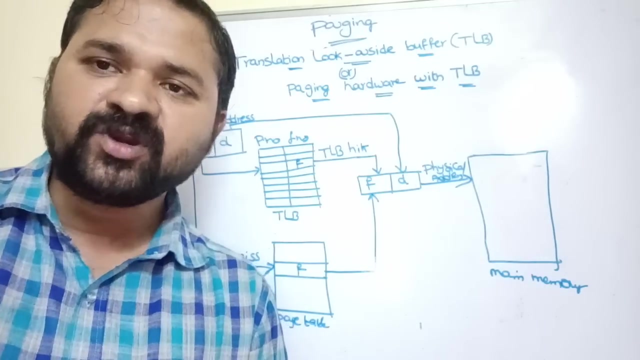 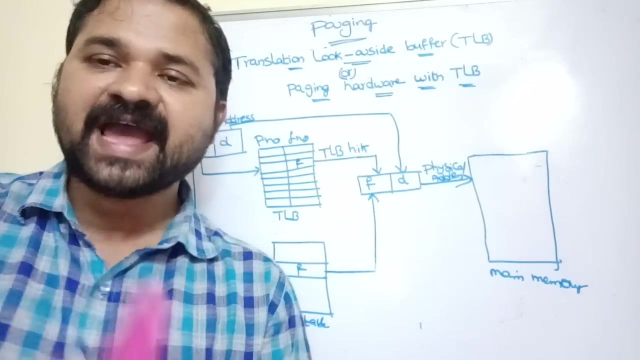 So in this way we can find out the physical address for the corresponding logical address. Now let us see. Now let us see about implementation of page table. So where we have to store page table, If we store page table inside a register, generally we know that registers are very, very faster than main memory. 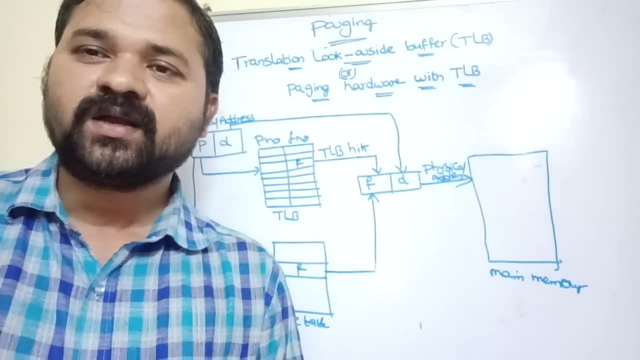 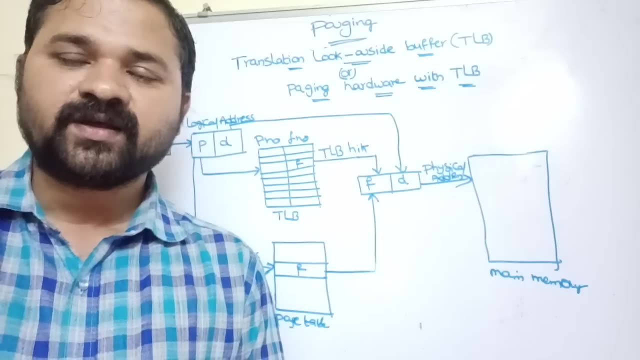 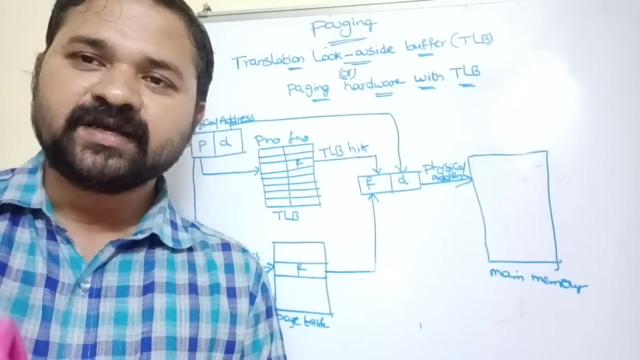 But registers are very, very smaller as well as very, very expensive. If we store page table inside a register, then we can access the data in a faster manner. But here the problem is the size of a register is very, very small. 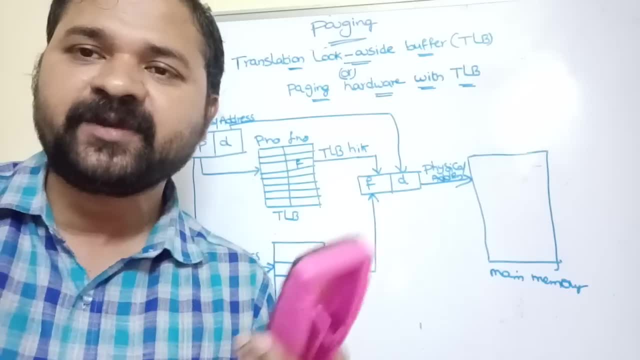 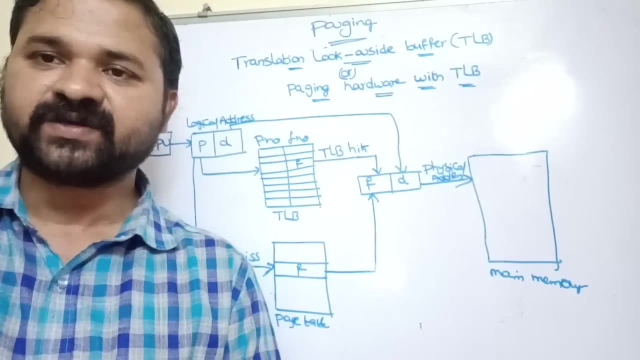 Generally, register size will be like 1 KB, 2 KB, 3 KB, like that, Whereas page table contains lakhs of entries, lakhs of pages. So it is not possible to store a large page table inside a register. 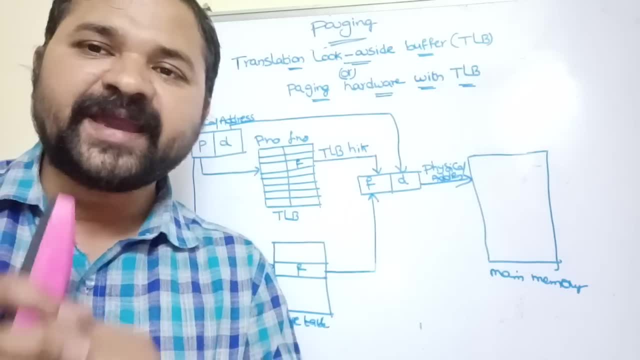 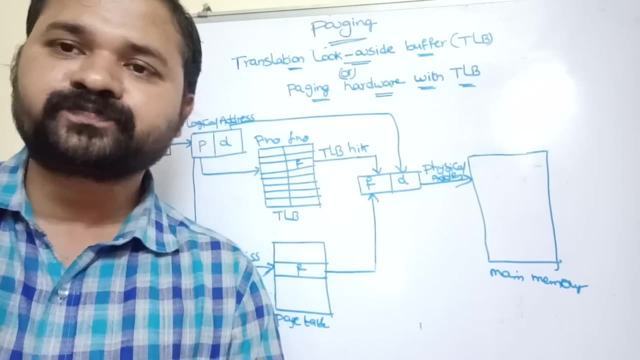 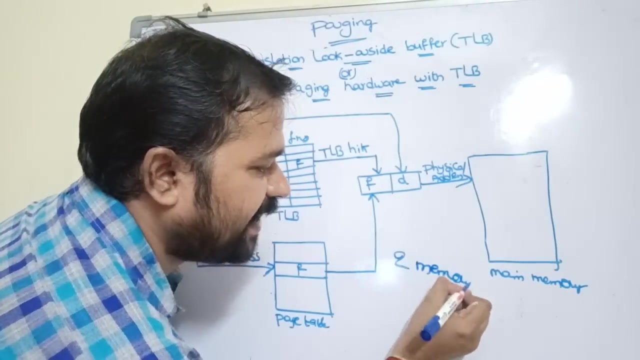 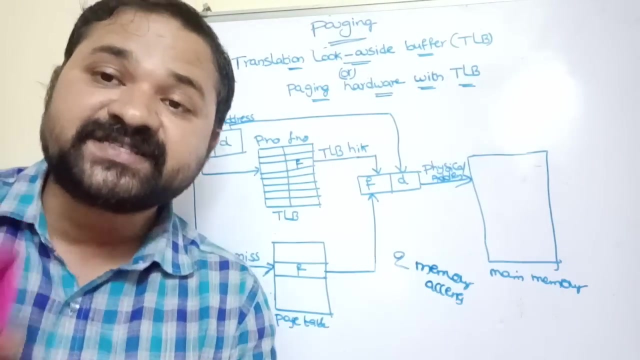 So that is why we need to store page table inside a main memory. If we store page table inside a main memory, then the problem is we require two memory accesses. We require two memory accesses for accessing an instruction, For executing an instruction. 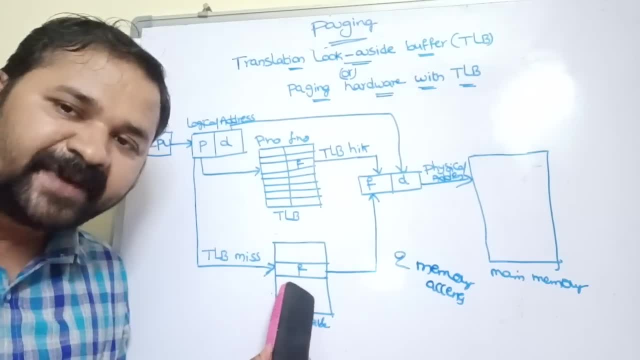 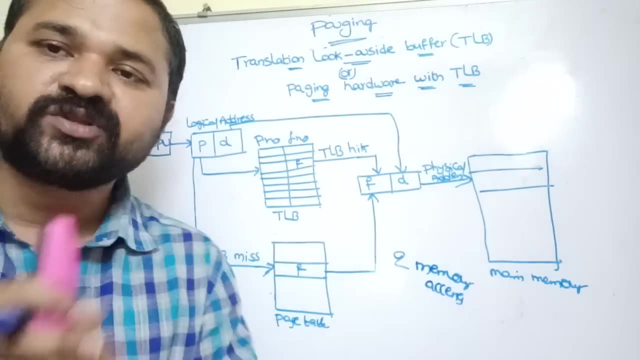 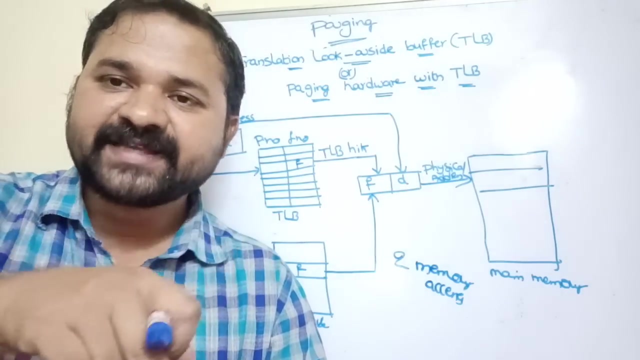 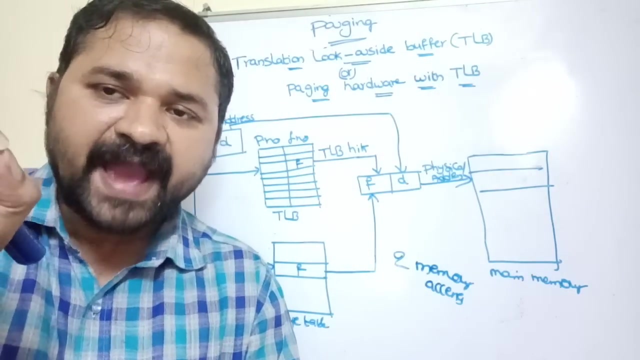 One memory access for accessing the page table, another memory access for accessing the main memory. we know that cpu generates logical address. logical address is divided into two parts. page number offset page number will be given as input to the page table. so in order to access the page table, 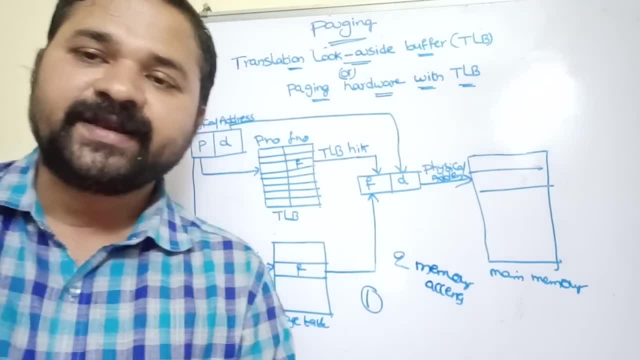 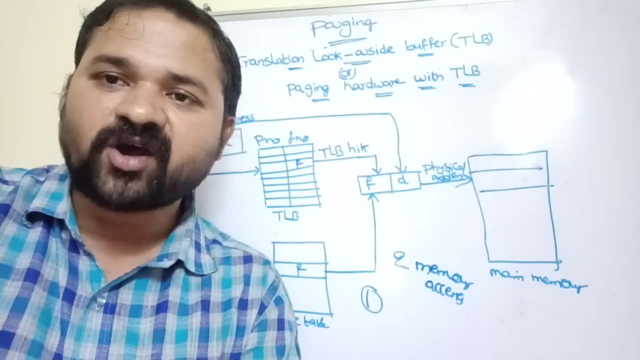 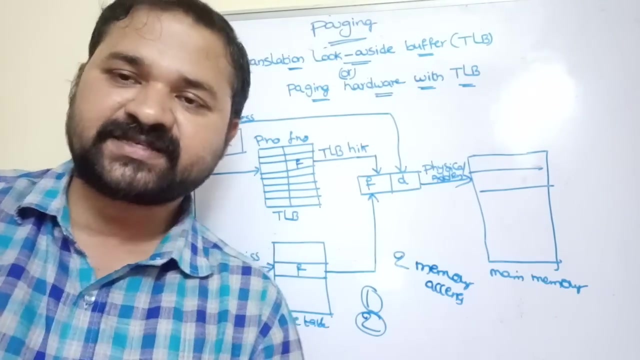 we require one memory access. next, if we combine frame number with page table produces frame number as the output. if we combine frame number with offset, it will use the physical address. so in order to access the physical address, we require two second memory access. so we need to have 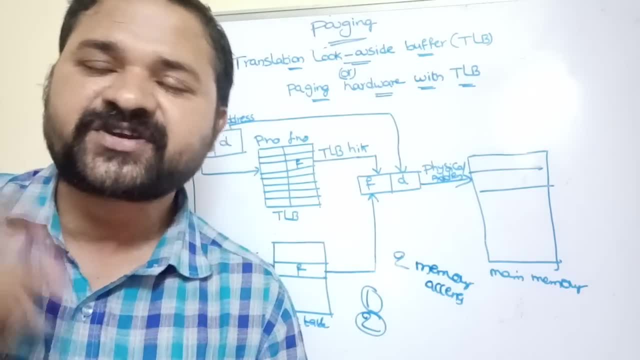 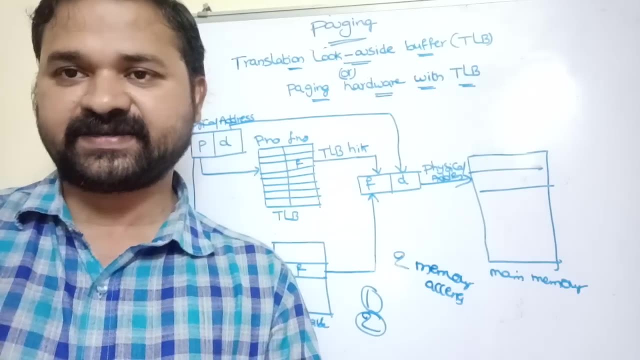 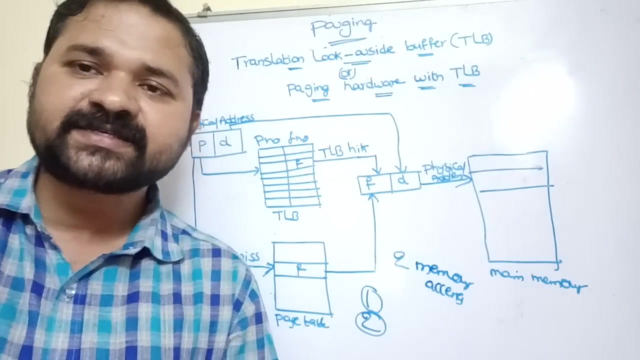 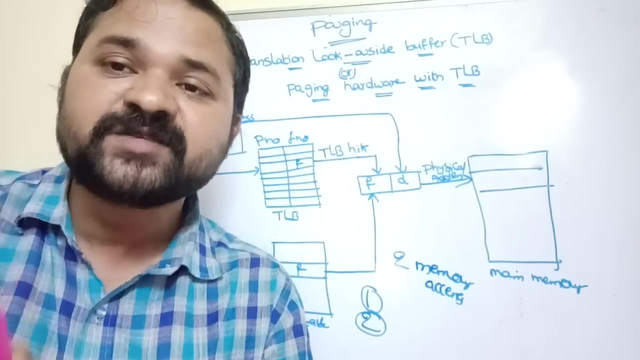 two memory accesses for executing a single instruction. so if we have lacks of instructions, then we need to have lacks of memory accesses. okay, so that is the problem here: for executing a single instruction, instead of one memory access, we need to have two memory accesses. so this is the problem here. so, in order to overcome this problem, 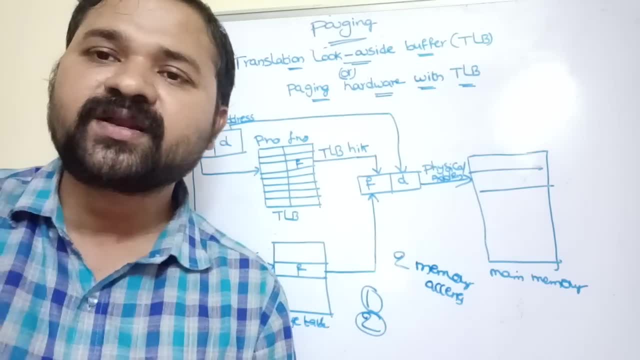 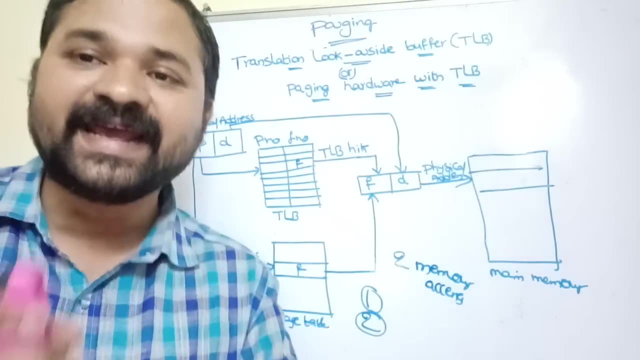 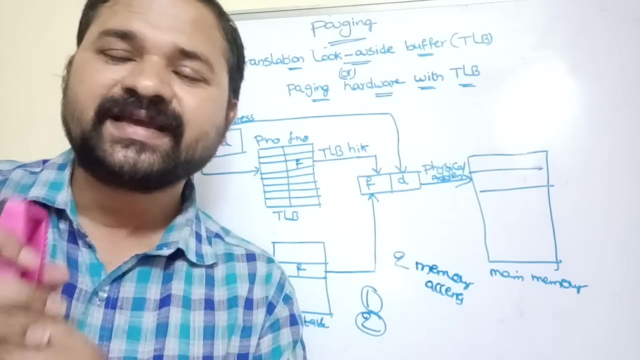 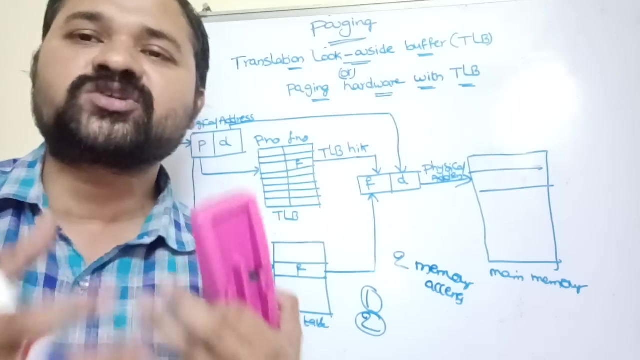 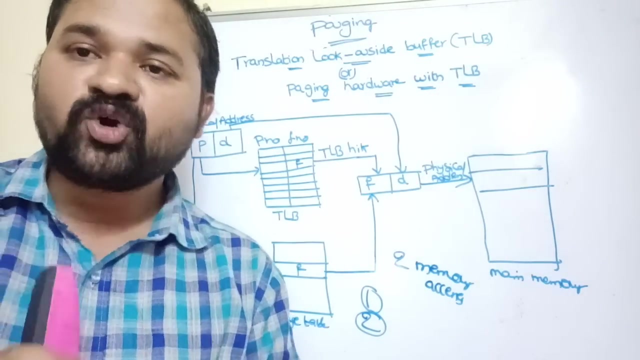 we use a faster, smaller catch called translation, look aside buffer. in short, we can call as tlb. tlb is a smaller, faster, special catch. here catch means it is not a catch memory- okay, it is a register only, but it stores large amount of data- okay. next, tlb is associative memory. we know that. 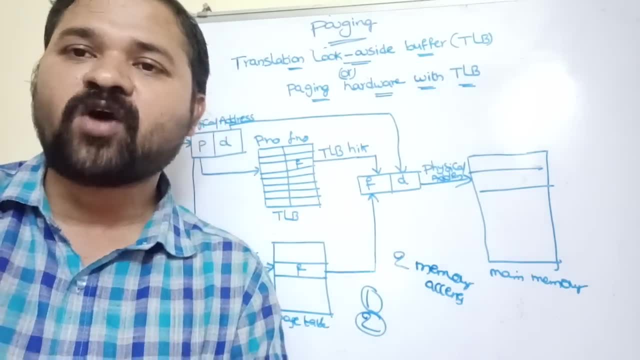 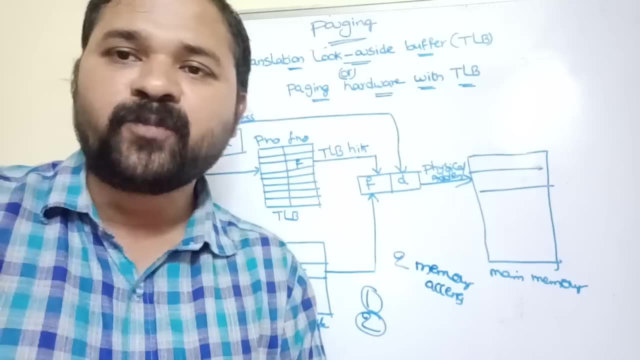 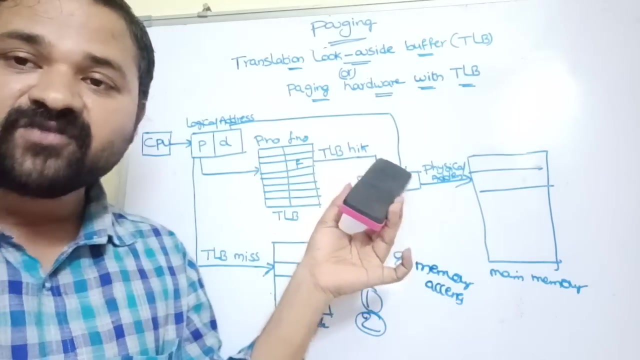 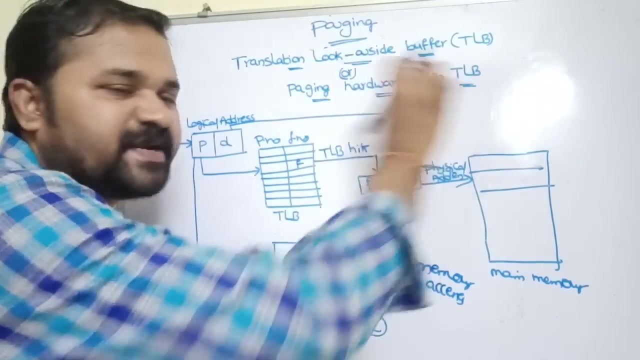 in associative memory, information is stored in the form of tags, where each tag is represented in the form of a tail. the first component of the pair is key. the second component of the pair is value. here key means space number, value means frame number. so let's see the diagram here. pacing hardware with translation. look as a buffer. now translation. 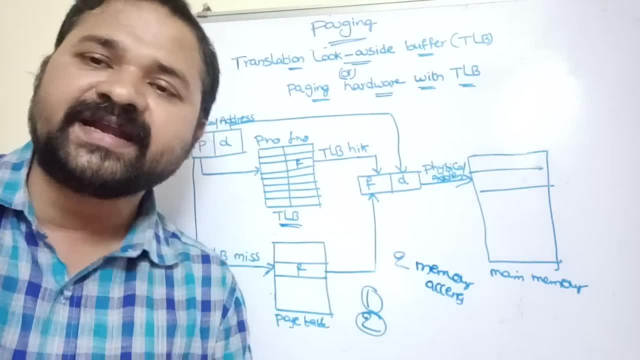 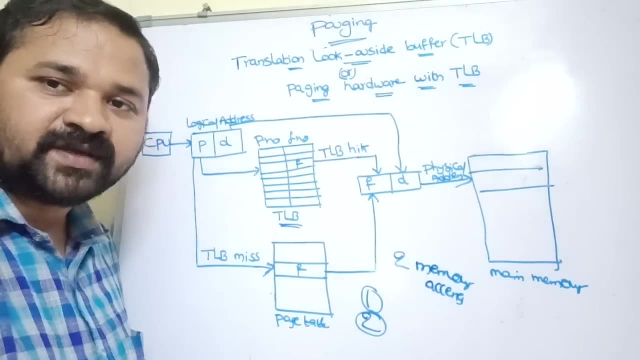 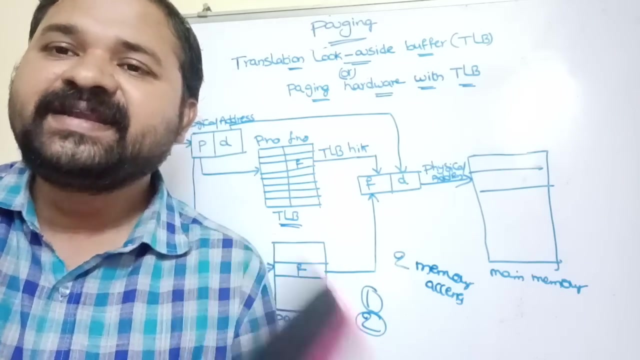 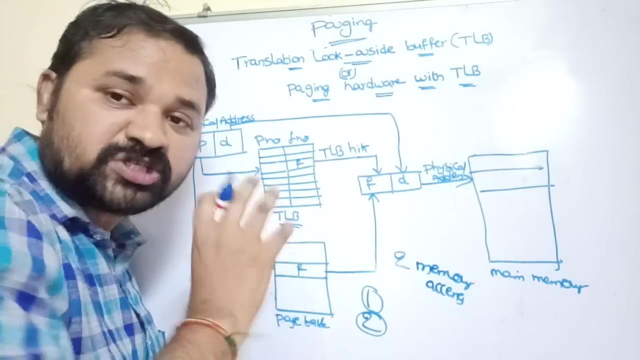 look, this is tlb. tlb mainly contains the frequently, the most frequently accessible entries of the page table. let page table contains thousand pages. out of those thousand pages, let we are accessing 10 pages very frequently, so dlb contains those 10 pages. okay, the free, the most frequently accessed pages. so, out of 100 pages, let us assume that we want to. 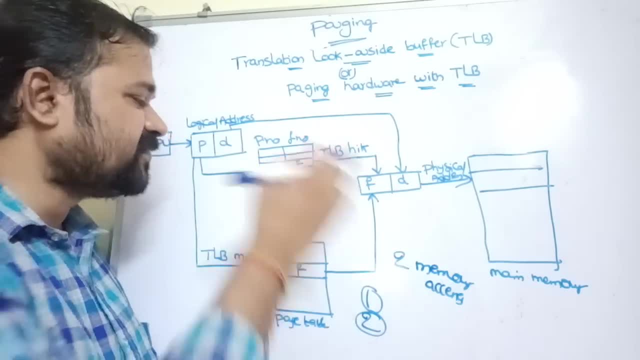 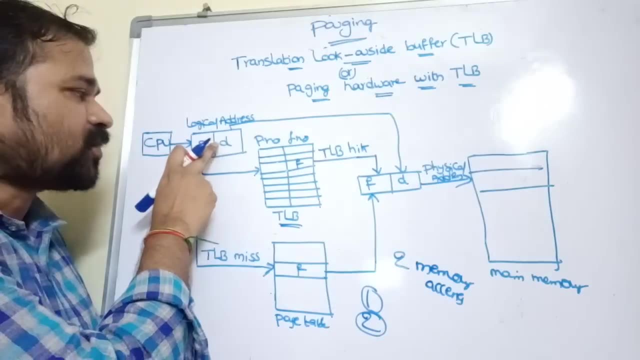 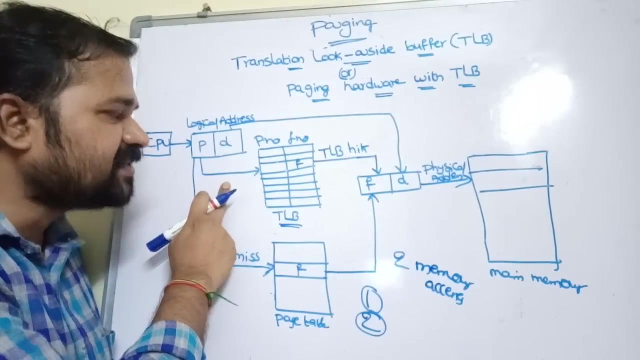 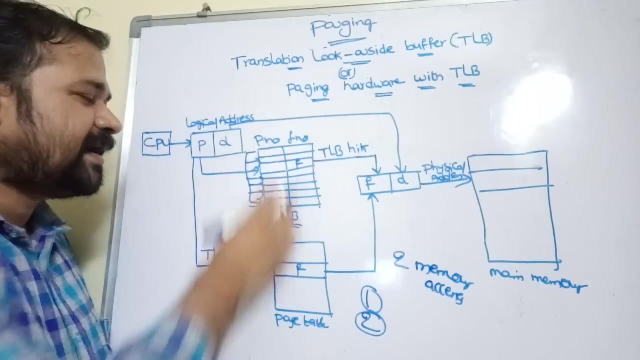 access five pages very frequently, so those five pages will be stored in the tlb. okay, so first cpu generates a logical address. that logical address is divided into two parts: page number offset. this page number will be compared with all the page numbers. okay, here this is tlb. so in tlb what will happen is every page number will be compared with this page number. 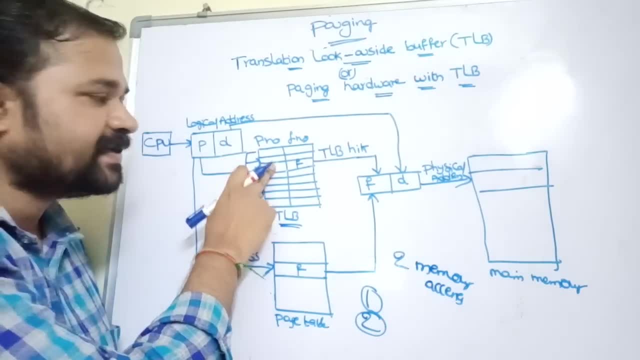 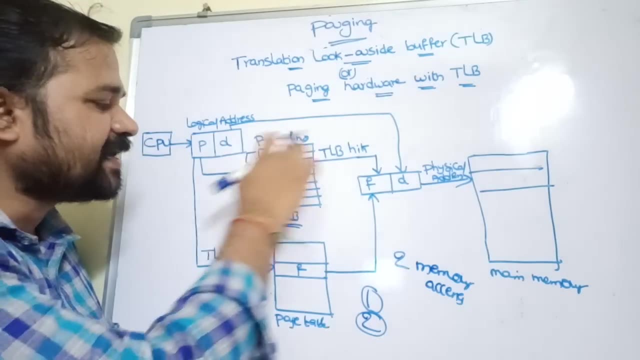 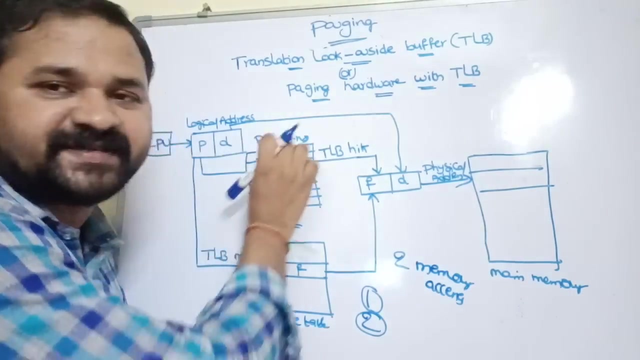 so if if there is any match found, then it will gives the corresponding frame number. okay, so what we are doing? we are giving page number as the input to the tlb. so in tlb, what we have happened, this page number will be compared with all the page numbers if there is a match found. 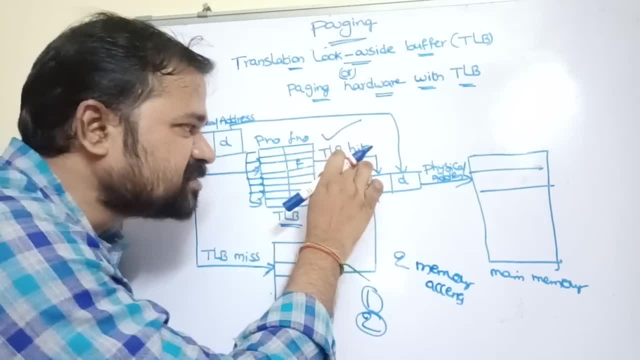 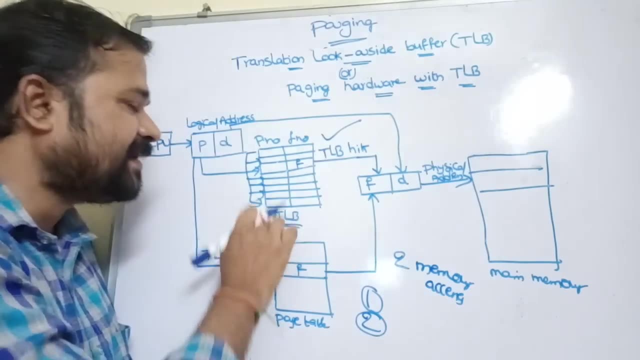 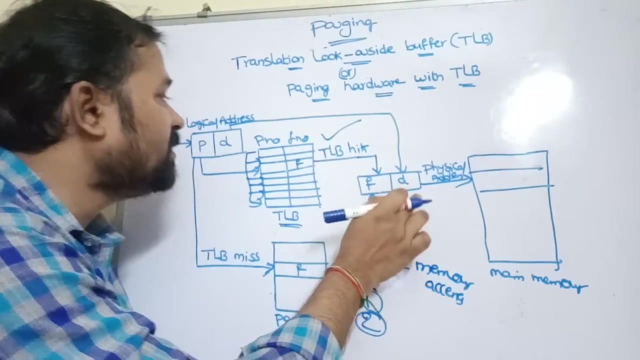 then it is called as tlb hit. so hit specifies that the corresponding page number is available in tlb. so tlb has two entries, two columns: page number, frame number. it gives frame number as the output. if we combine frame number with this offset, it will use the physical address so we can access. 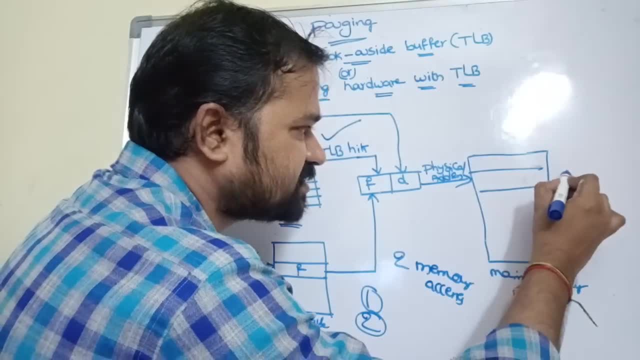 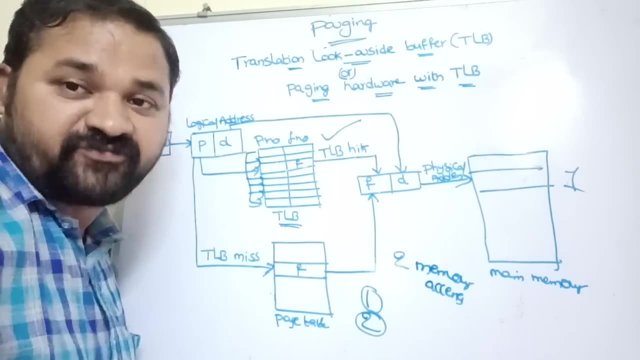 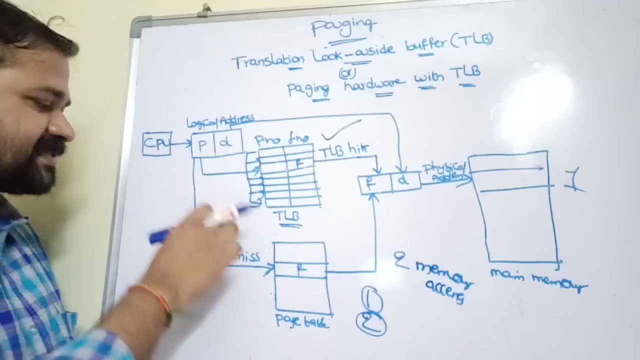 the instruction in a faster manner. here also, for accessing the instruction we need to have one memory access, but here this tlb is very, very faster than the if paste table resides in main memory. okay, so that that instruction will be accessed in a faster manner. next, if page number is not available, 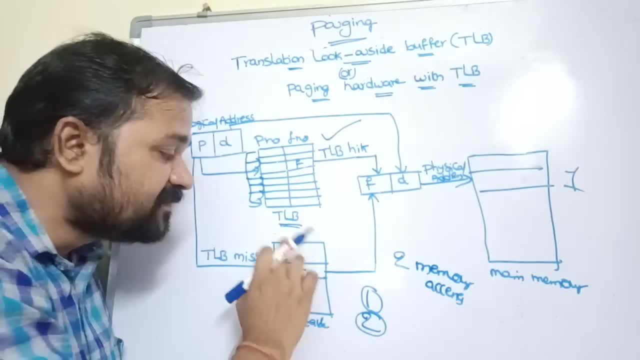 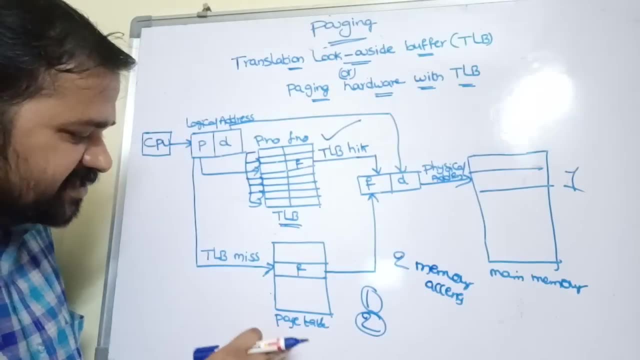 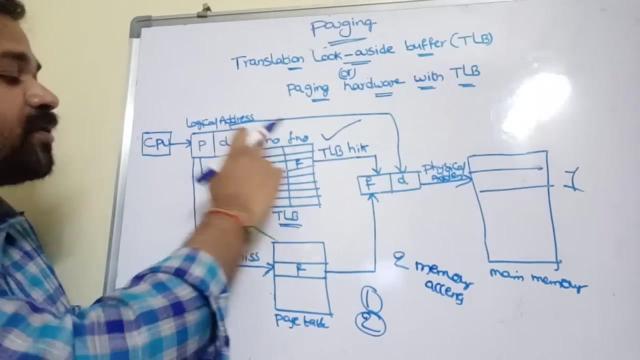 in tlp, then this page number will be given as input to the paste table. this space table resides in main memory only. okay, so pasteable. this is called as tlb miss. so tlb miss means the corresponding base is not available in tlp. okay, so base table accepts base. 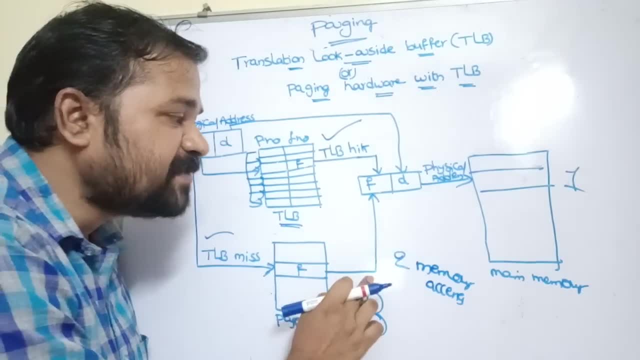 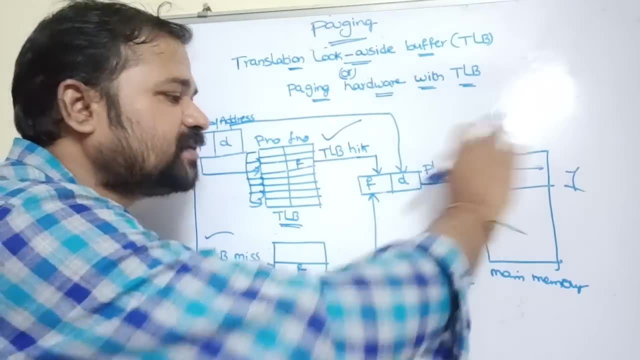 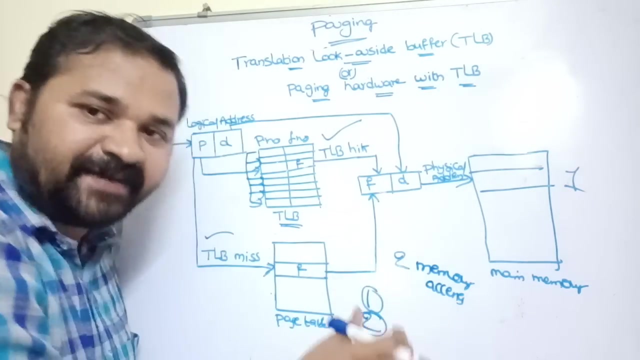 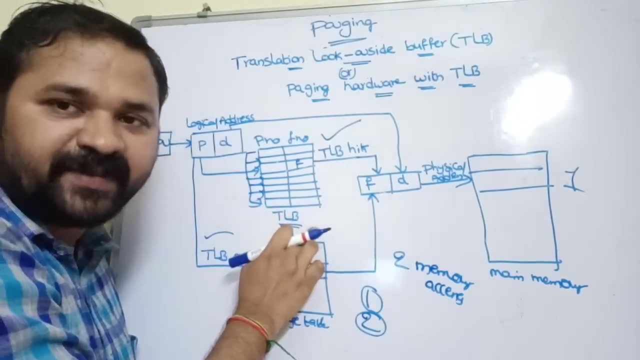 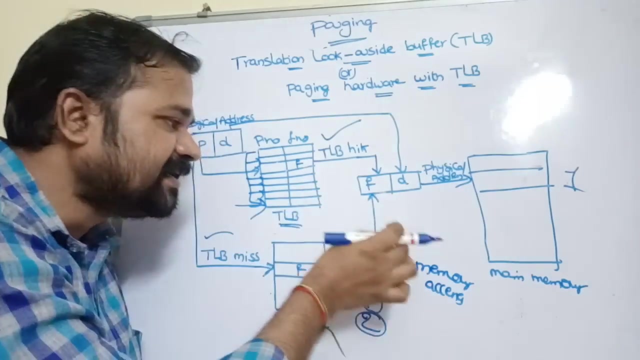 number as the input and produces frame number as the output. if we combine frame number with offset then it will give the physical address so that cpu access that instruction here. after getting frame number, the corresponding entry- that means the page number and frame number- information will be updated in tlb, suppose if tlb is full then one of the row will be replaced with this new row. this: 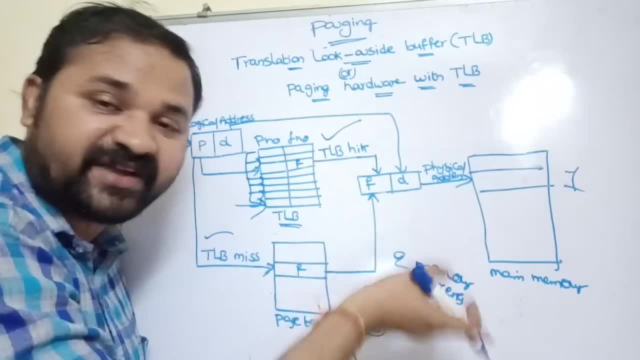 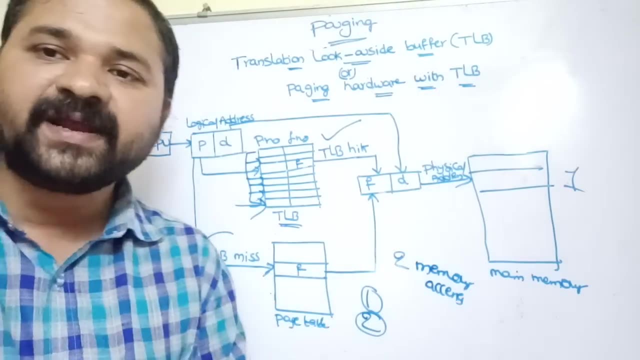 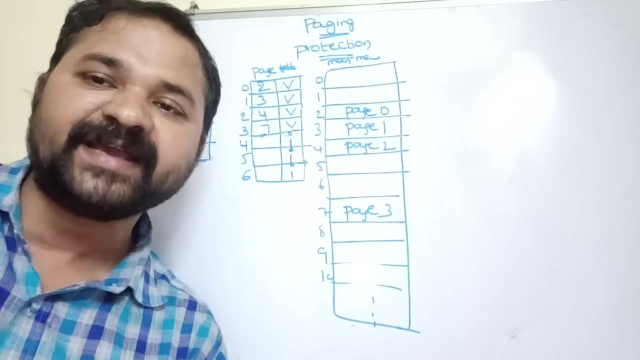 new row contains what page number and column, page number and frame number. okay, that for replacement. we have several replacement algorithms. okay, so in this way we can implement tlp. now let's see how to provide protection in pacing. so this is our process. this is page table. 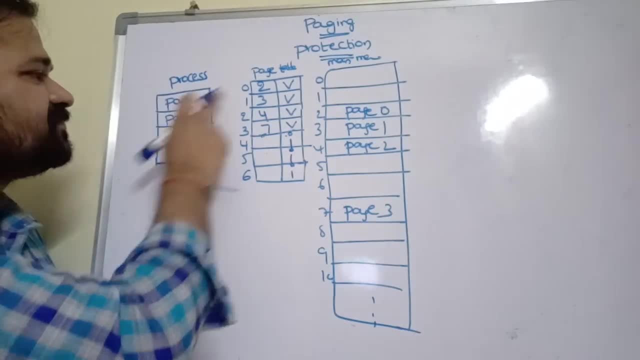 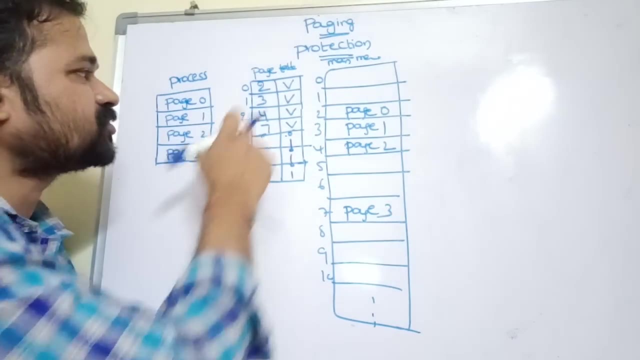 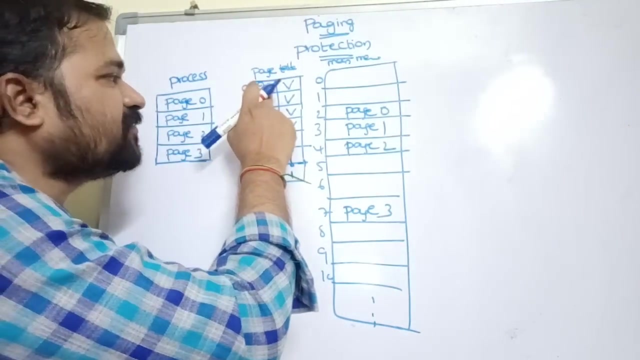 and this is main memory. so this process is divided into four pages and this is space table. so page table accepts page number as the input and produces frame number as the output. so the first row specifies that page number 0 is available in frame number 2. so in frame 2 we have 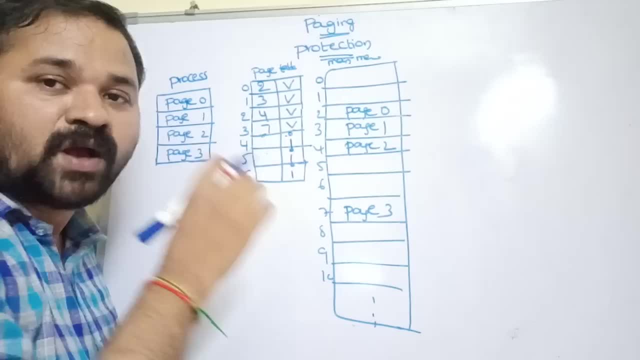 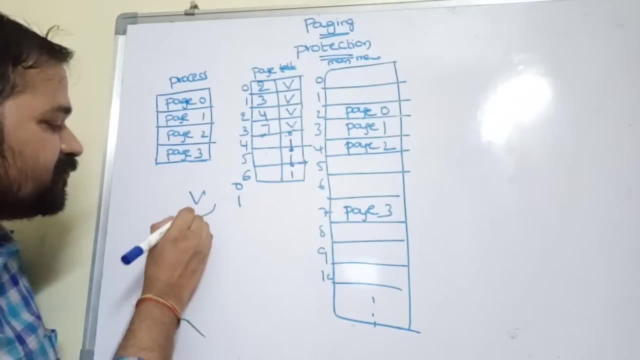 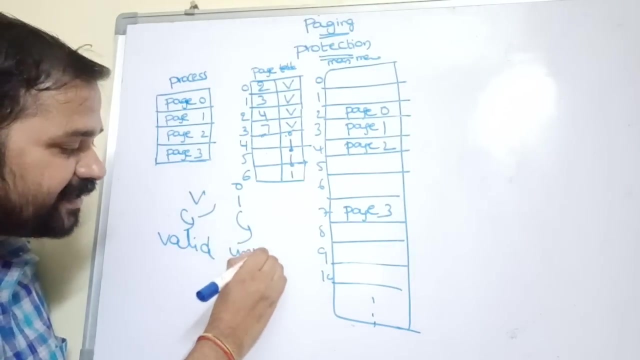 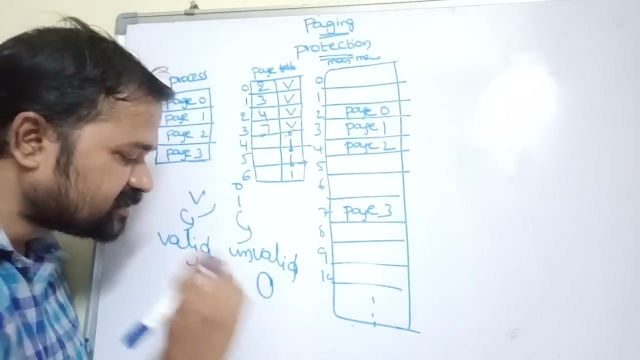 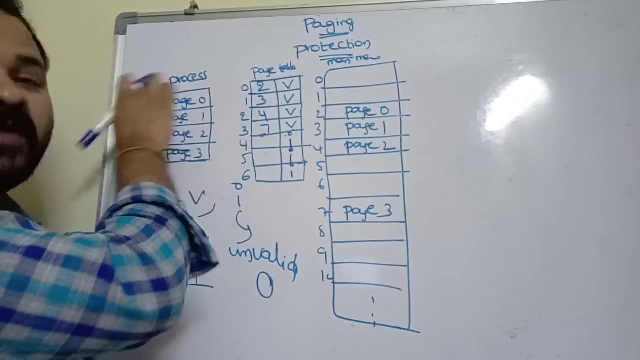 page 0. here the protection bit is operating system. provide the protection bit with the help of v or i, where b stands for valid bit whereas i stands for invalid bit, or in place of v we can use one. in place of invalid, we can use zero, so valid, or one specifies that the corresponding page is. 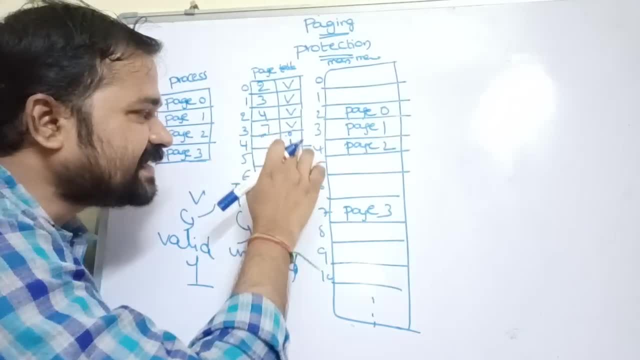 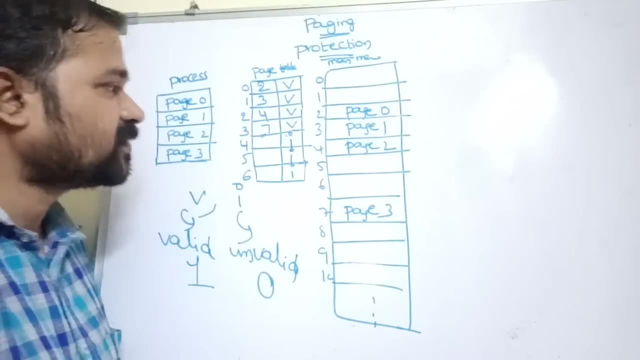 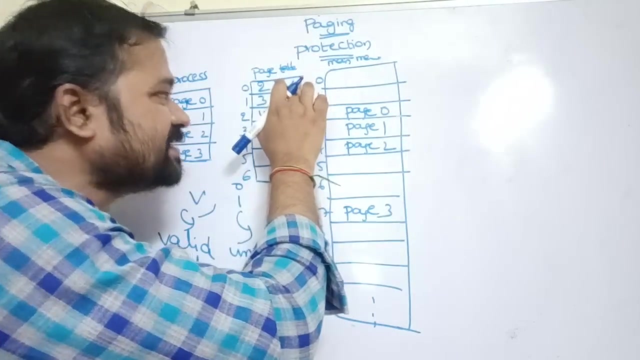 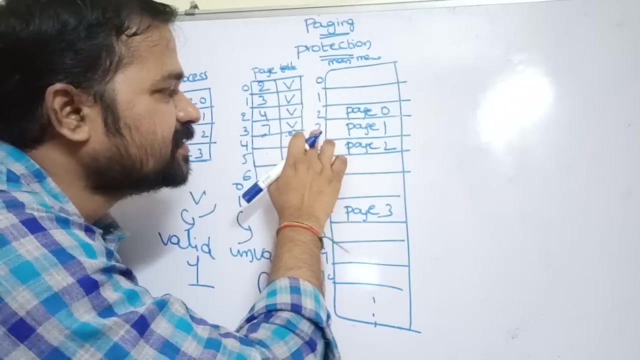 belonging to the process, whereas this invalid specifies that the corresponding page number doesn't belongs to the process. so here page number 0 is belonging to the process. so here the production bit is v. next, the second row specifies that page number one is available in frame number three. so in frame three we have page one. so 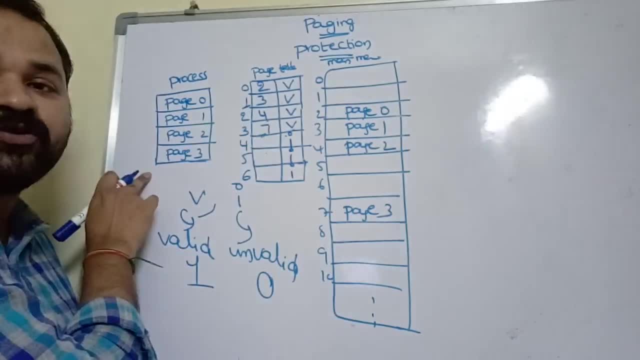 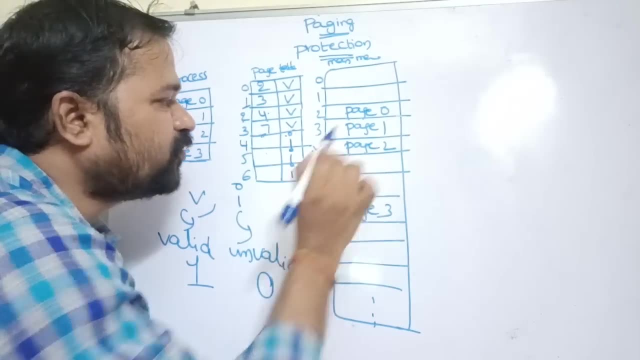 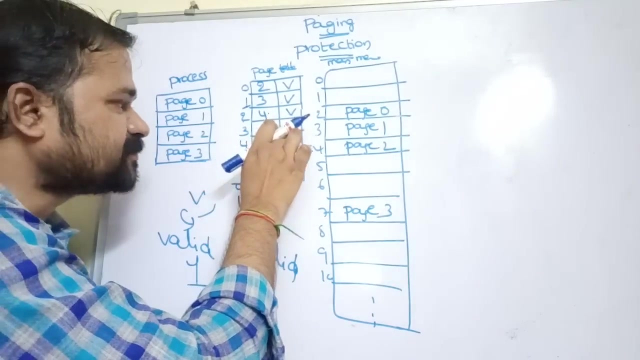 this v specifies that this page one belonging to the process. next, this row specifies that page two is available in frame four. so in frame four we have page two. so v specifies that this page number two is belonging to this process. next to this v specifies that this page number three: 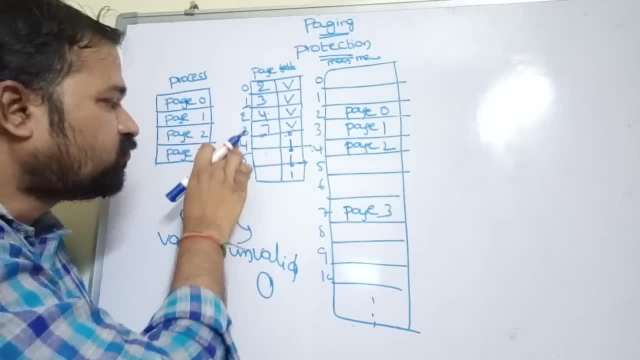 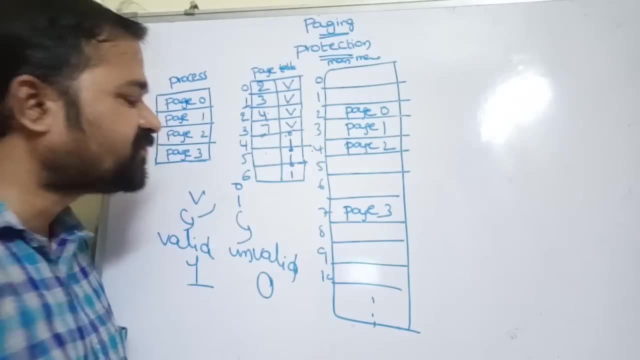 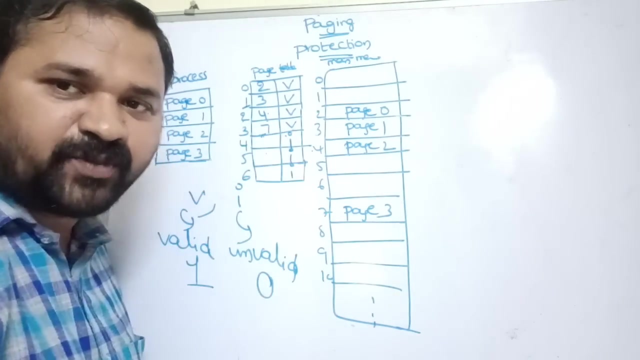 is belonging to the process. if you take four, five, six. four, five, six are no longer belonging to the process. so here the production bit is i, so i stands for invalid bit. so these processes doesn't belongs to the process. so while creating the page table, if the corresponding process is belonging to 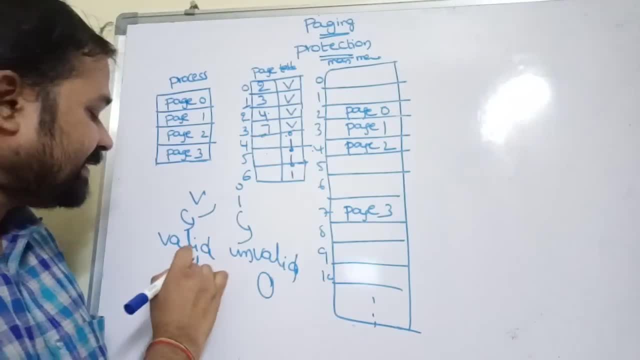 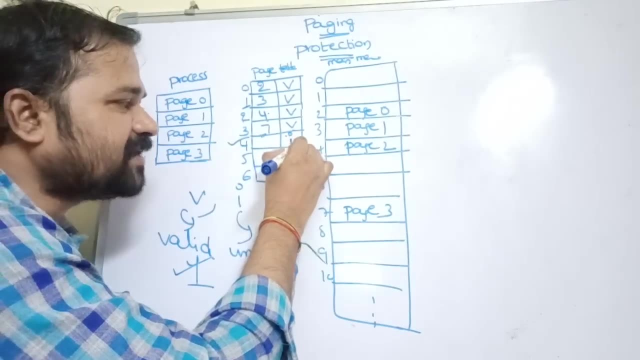 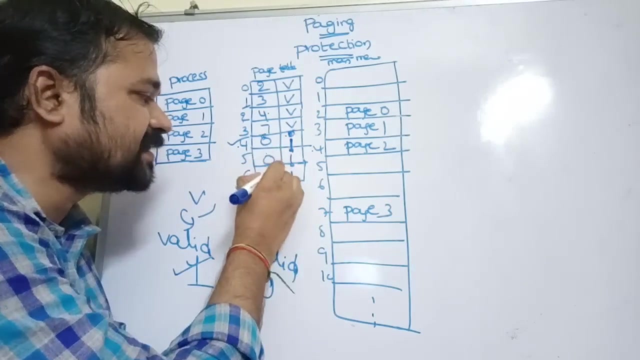 the process, then production bit means v or it is set to one. okay, so if the if cpu needs to access fourth page, then automatically here we have a invalid bit. so what will happen? cpu doesn't access this page, even though some frame number is available here, even though some frame is specified. 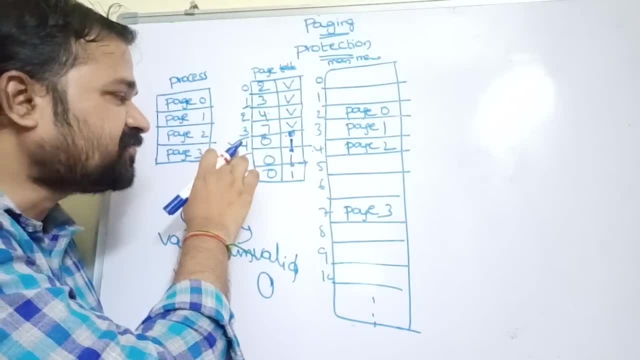 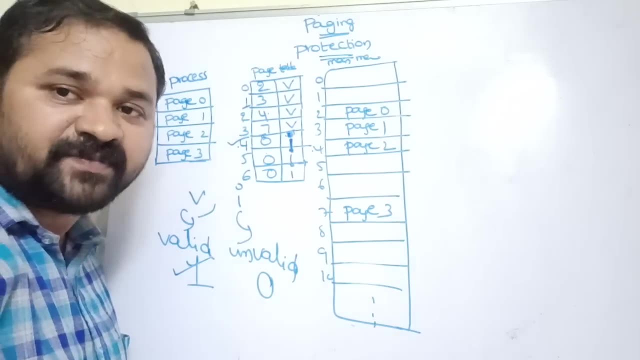 let us assume that some statements are like this. it specifies that page field, page 4, is available in frame 0. but here what is the production bit? here i i means invalid bit. invalid means this space 4 doesn't belongs to the process, so cpu doesn't execute this process. 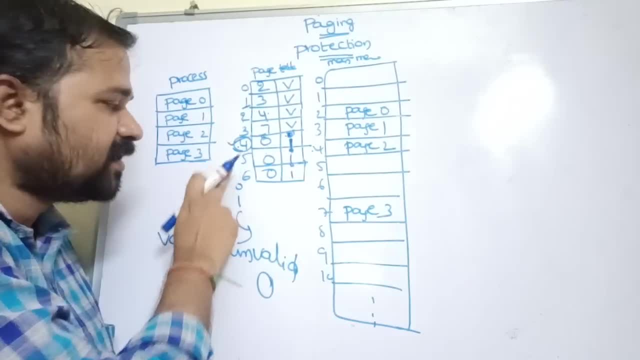 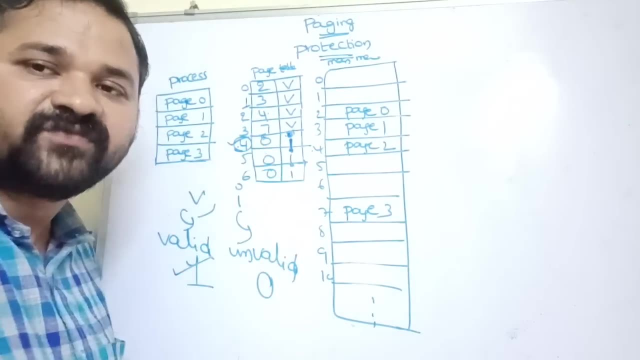 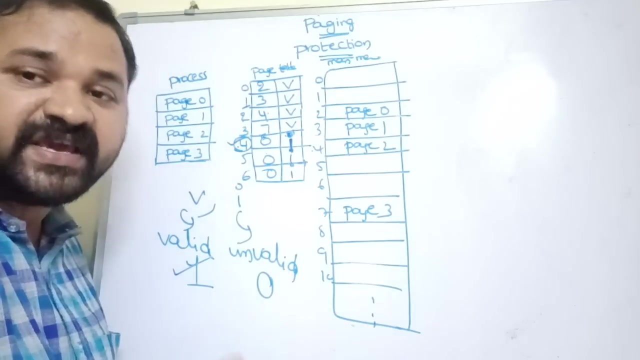 likewise cpu doesn't execute this page number. likewise cpu doesn't execute this page. why? because these three production bits are i, so in this way we can product, provide protection mechanism for the pacing environment with the help of a protection bit. v are i, so v means protection is set, that 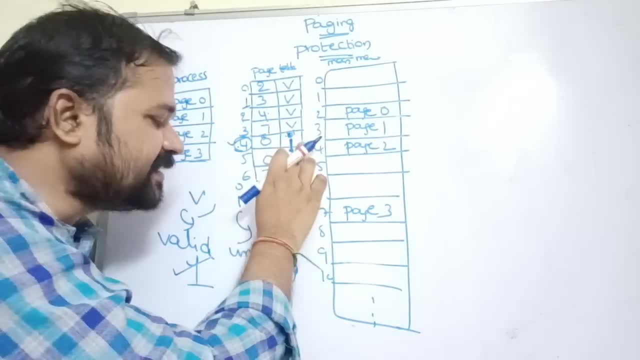 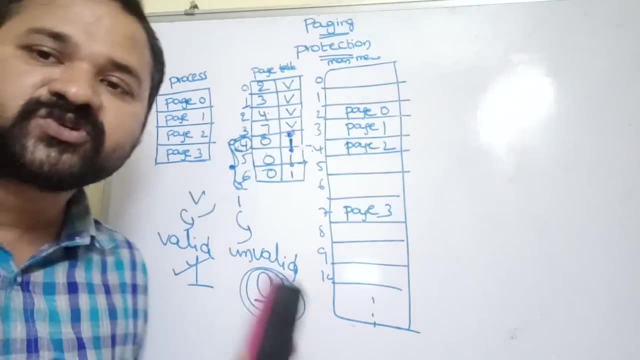 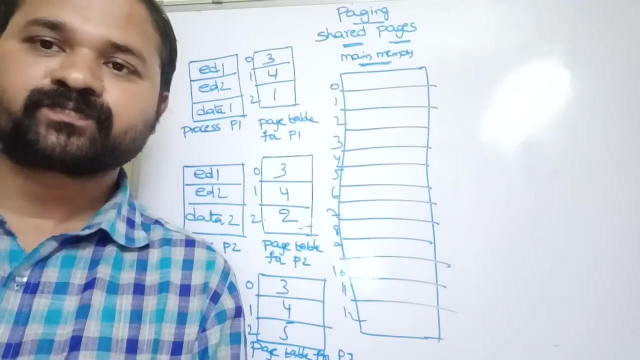 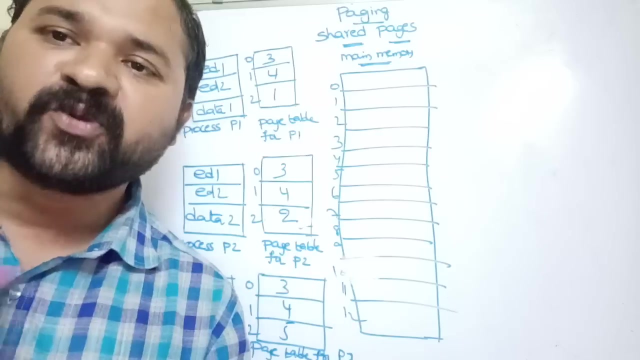 means that page number is belonging to the process. i means it is zero. that means there is no protection. that means this is this space is doesn't belongs to the process. one of the advantages of pacing is shared pages. in a multi-programming, multiple users can execute multiple processes by sitting at different computers. let us assume that. 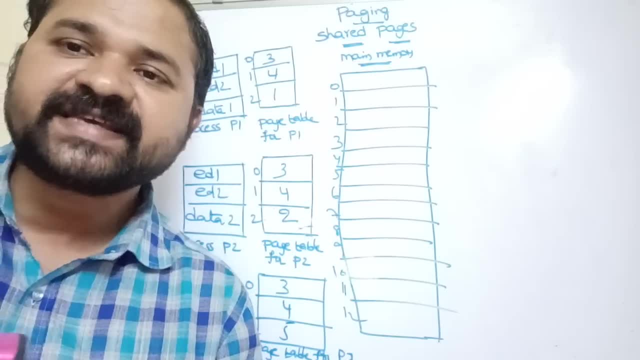 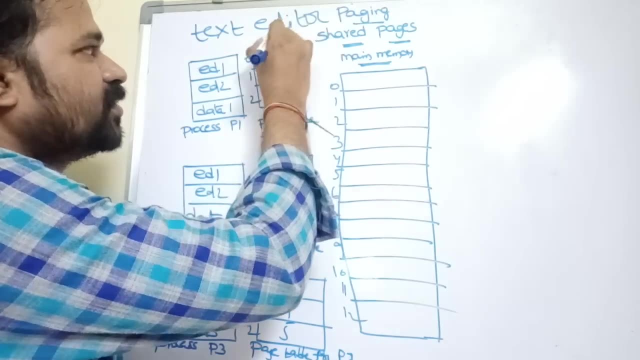 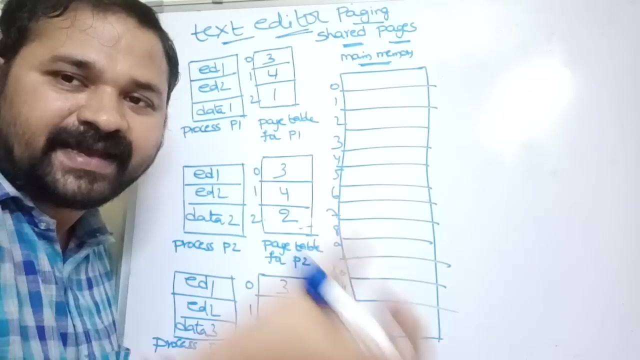 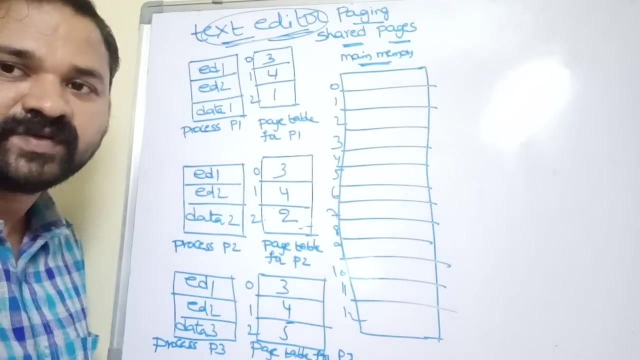 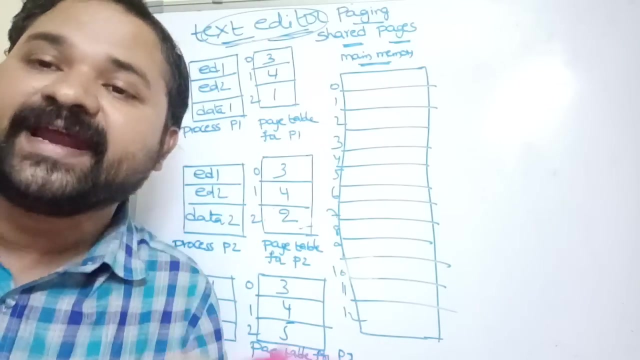 there are three persons who are working on the same application called text editor. let us assume that three persons wants to make use of text editor. so instead of using text editor at three computers, what we can do is we can share this text edited page. so this is nothing but shared pages. here, each process has its own data and its own resistance. 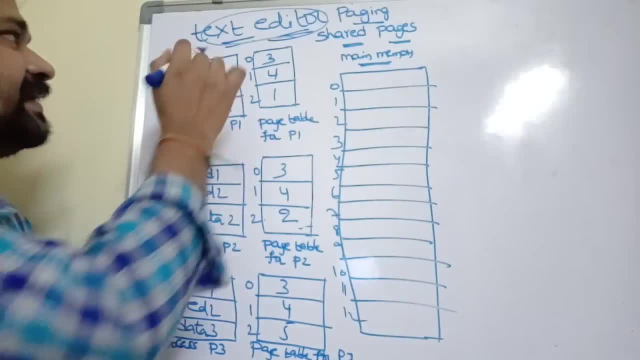 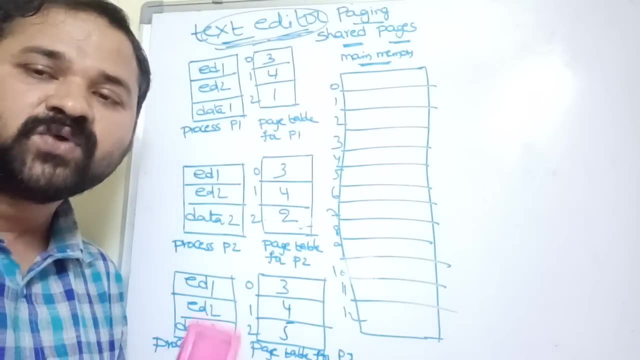 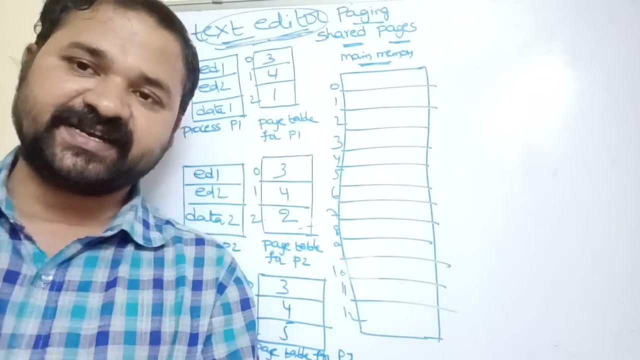 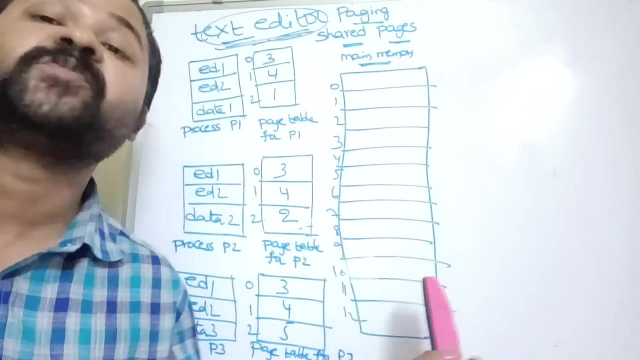 but all the processes needs to use text editor. let this editor is read only code read only means only we can read the data from the application. it is not possible to make any modifications on the text editor. so here, the text editor is an application which is shared by three processes. 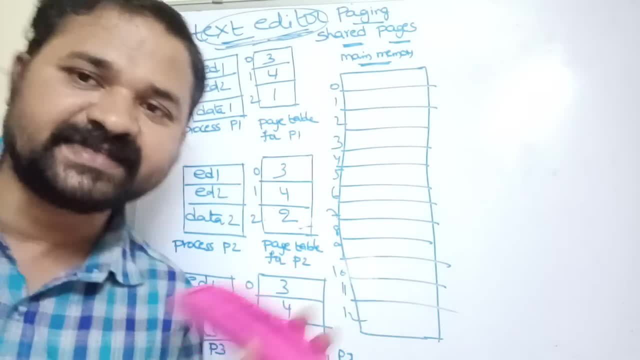 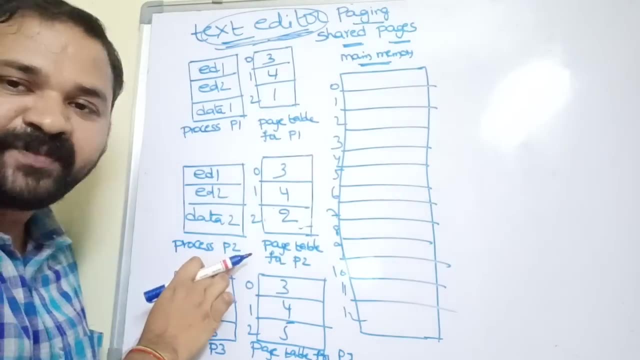 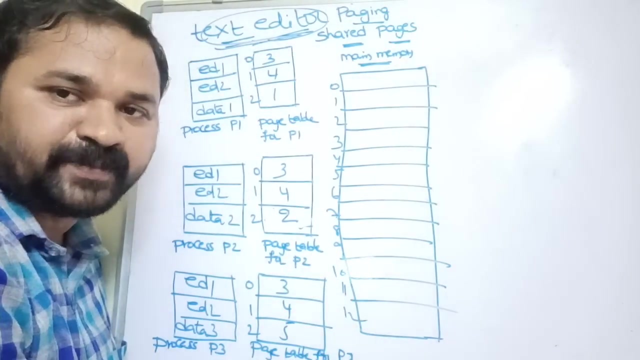 and each process has its own data. let's take this example. so this is process p1. this is space table for p1 process. this is process p2. this is space table for p2. this is process p3 and this diagram is for page table for p3. here let us assume that in text editor we have 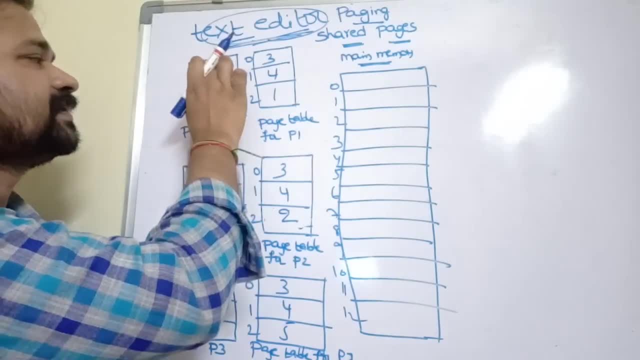 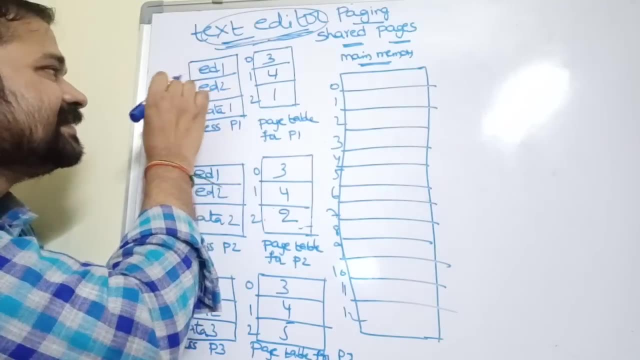 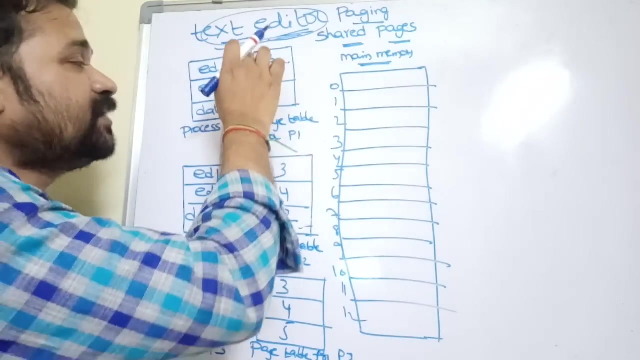 two pages, so ed1- ed2, ed1- ed2. so these two pages are belonging to the text editor, so we have to use these two pages in all the three processes. okay, so what is the paste table here? paste? we know that paste table accepts base number as the input. 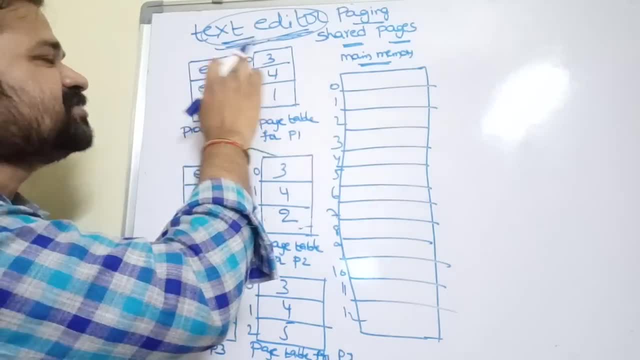 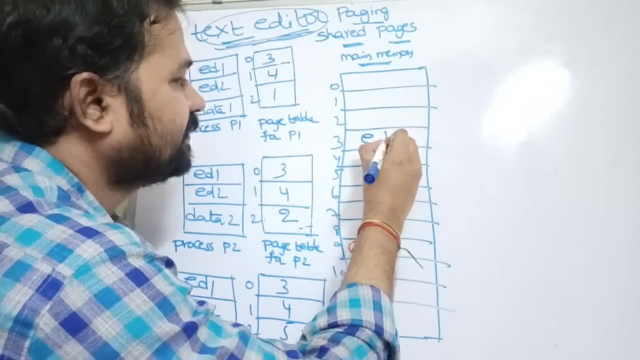 and it produces frame number as the output. so here page 0 means ed1, ed1 is available in frame 0, case 0 and factory 0 card detachable about ub'moment audio. so in frame 3 we have ed 1, deficit etc. 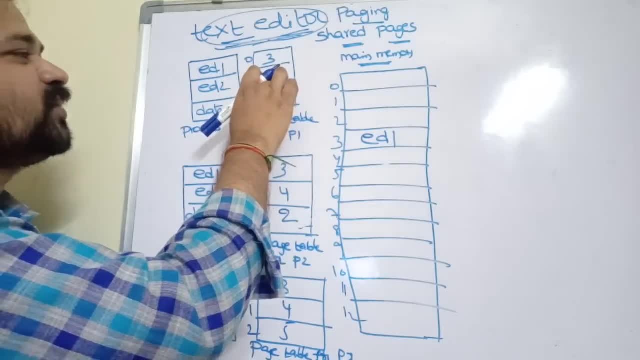 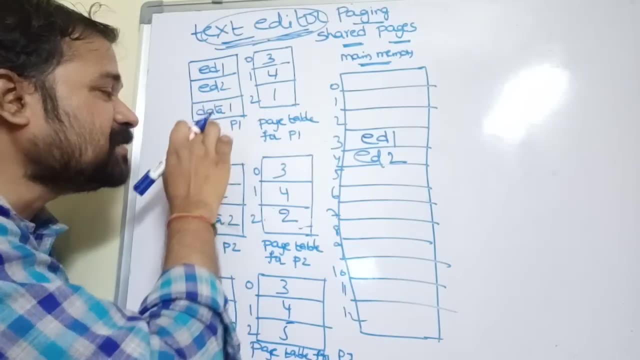 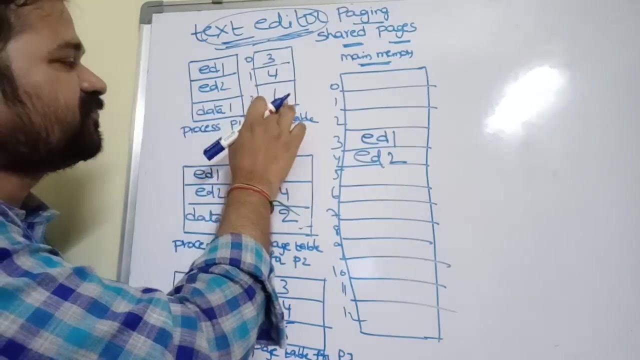 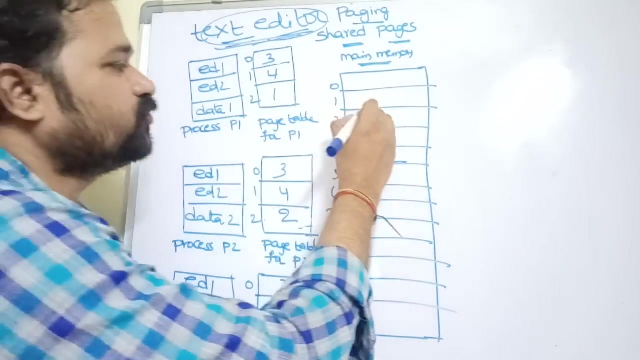 number one is available in frame number four. so in frame number 4 we have ed2, next data 1. so this data one is nothing, but p1 won't data, p1 won't application. so here, what is the frame number for page number two? frame number one. so in frame number one we have page two. so what is space two? data one, okay. 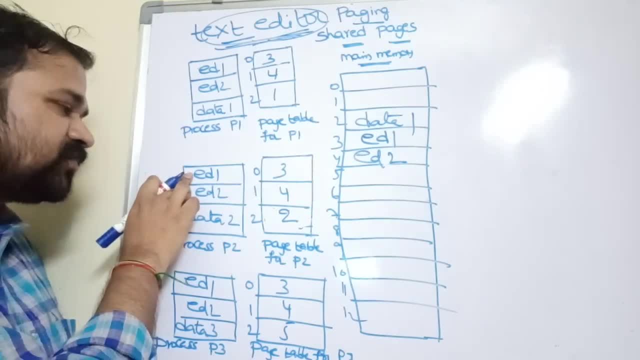 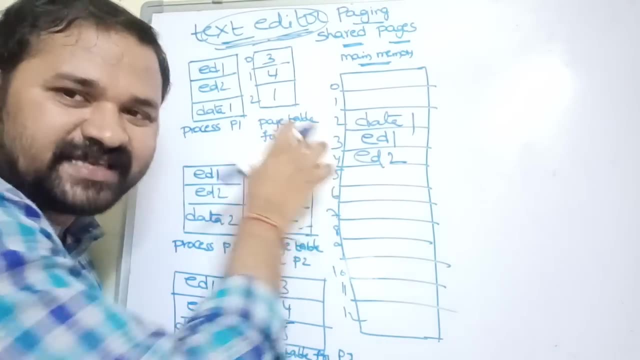 next, if you consider the second process, so in this process also we are using text editor application ed1, ed2. so zeroth page is available in page number three, so there is no need to store one more time. so already we have that page number and corresponding frame data. next page number one. 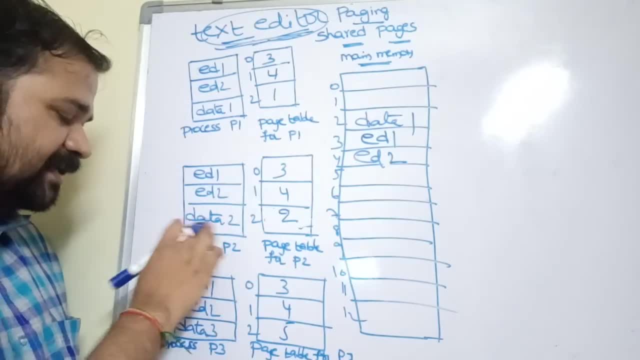 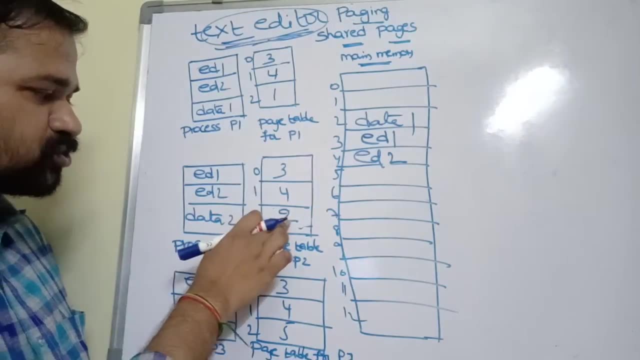 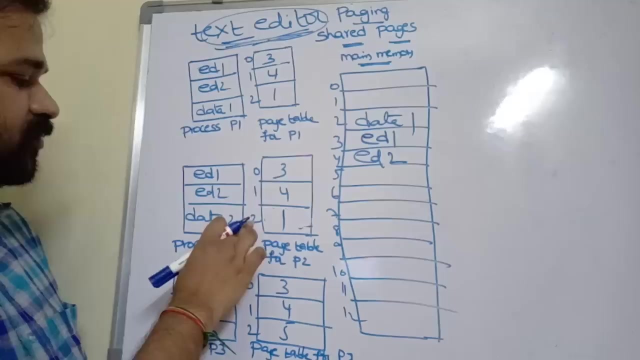 means frame number four. so already four contains cd2. next, this data two is nothing but process p2 won't application, process, p2 won't page okay, so we have to store in separate frame card two. so already we have assigned two, so let us assign one here. so here page number two is available in. 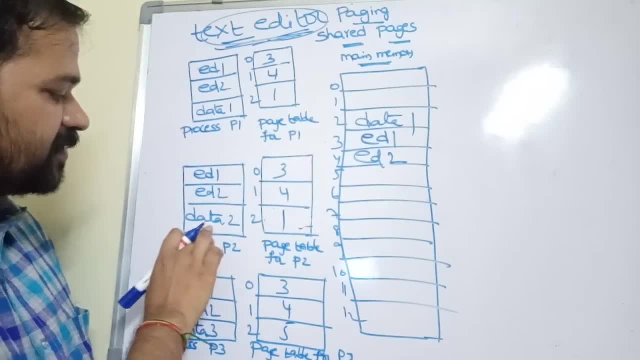 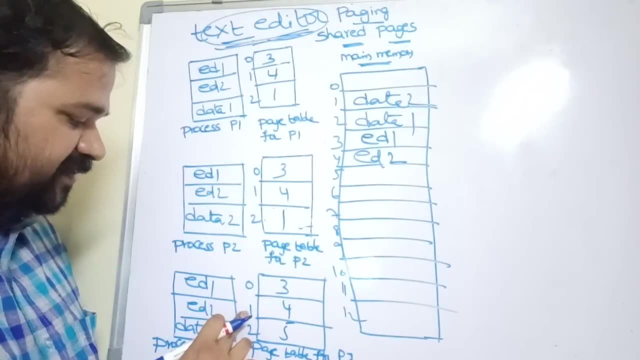 frame number one. so this is frame number one. so in frame number one store data two. next, if you consider the third application, so in page zero and page one we have page number zero is available in frame number three. so three, four means cd1, ed2. next page number two.